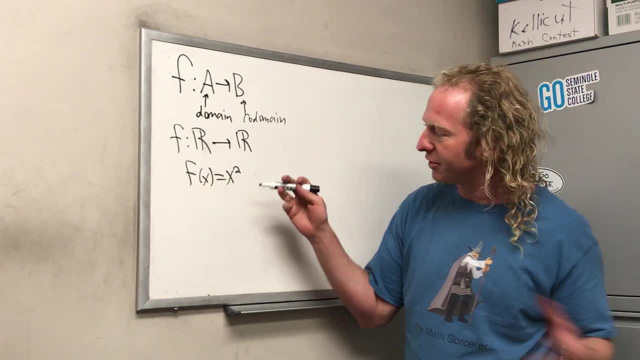 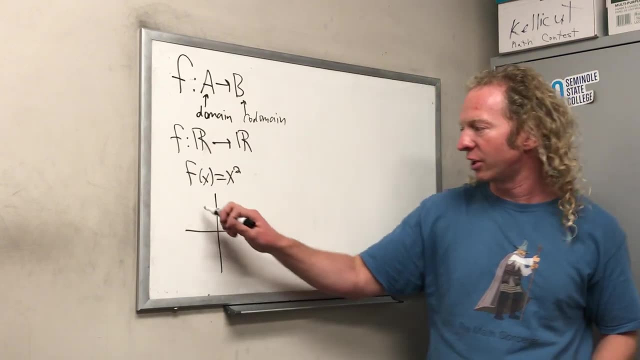 and then it squares it right. This is pretty cool. It's pretty cool. So let's think about the graph of this function. So if you graph this, what is the graph of X squared? Do you all know Parabola? It's a parabola, right, So it looks like a U. So 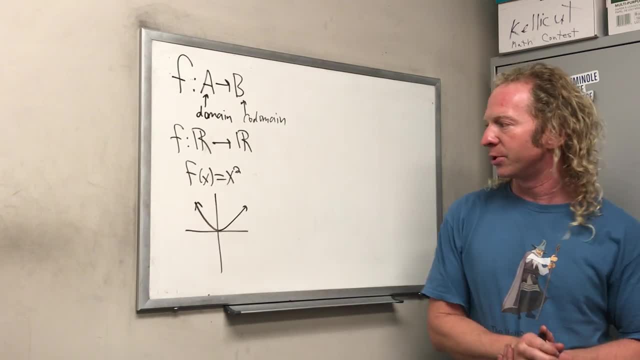 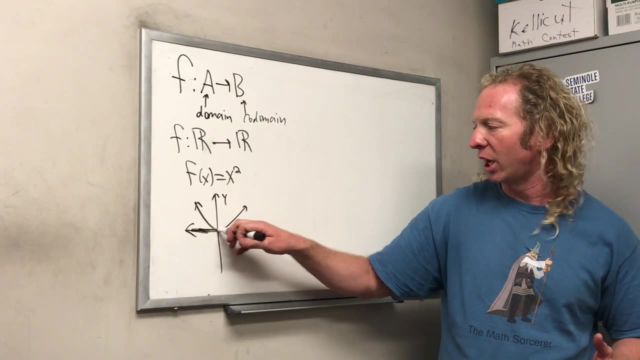 it looks something like this: right? So it's a parabola. So clearly, the domain is all the X's, It's all the inputs, right? So you see it's the entire real line, right Again. this stuff is super useful. You can know all the math in the world, but if you don't know this, 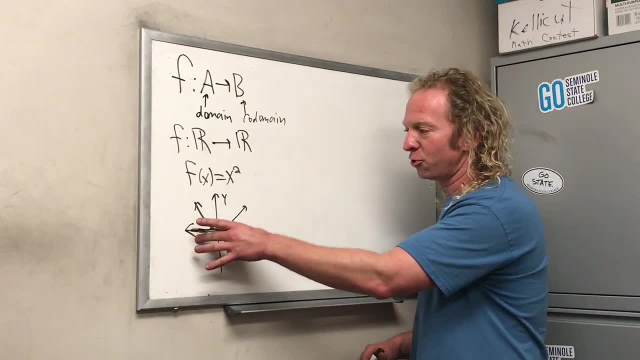 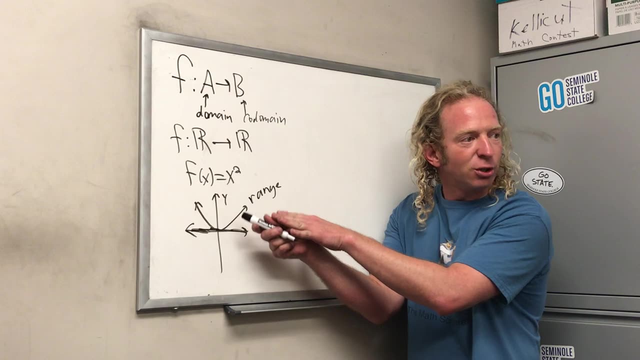 it's like: ugh, You need this for all high level math. So that's your domain. You'll notice something, though: There's a word for it. It's a word for it. It's a word for the range. The range is all the Y values, and you go from the bottom up: What's the? 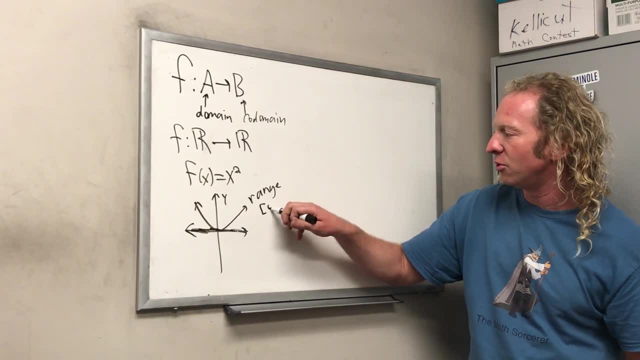 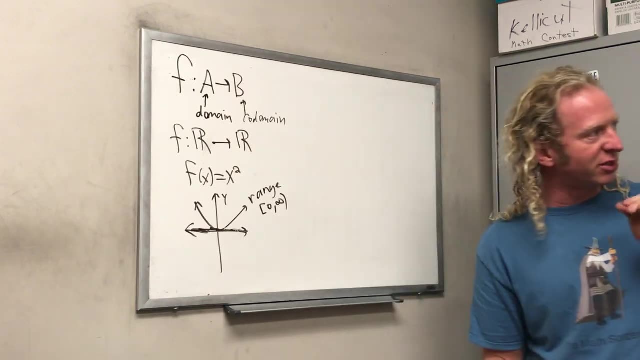 smallest Y value here, Zero. So it would be zero to infinity right. So that would be the range in this case. You'll notice the range is different from the codomain right, So it's different. I used to have this teacher. He was really, really good, He actually went. 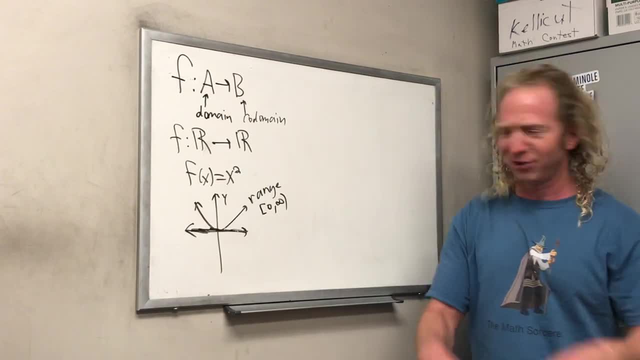 to Harvard and Brown and stuff. He was like: we don't use range in my classroom. I think I was like a legend, But why? Because range doesn't typically, I don't know. Range can mean a lot of things in mathematics. 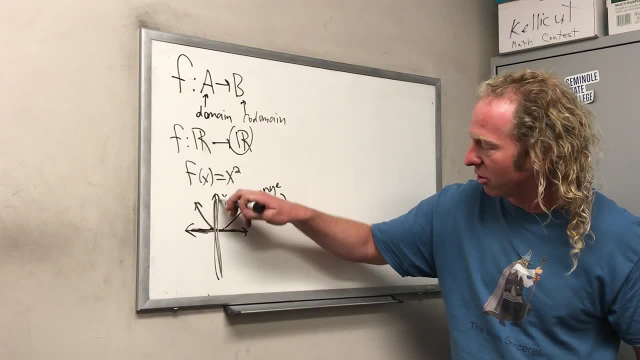 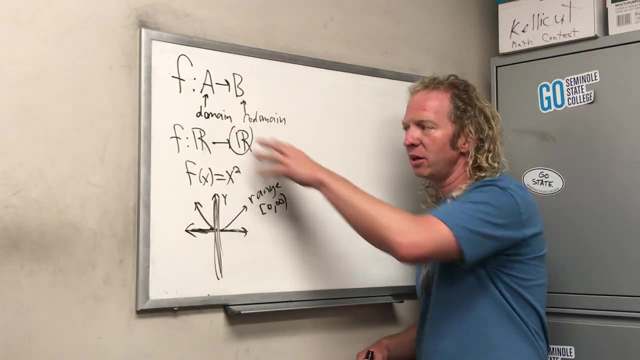 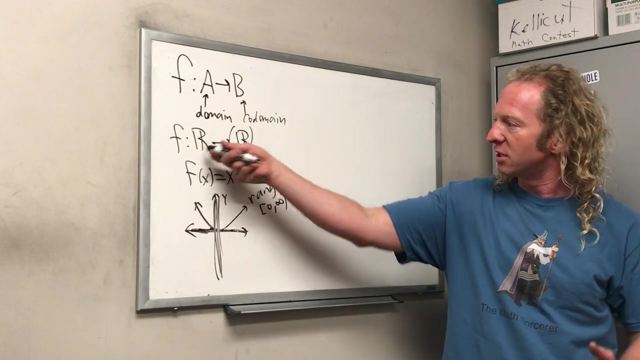 So codomain would be all of this right. So the range is a subset of the codomain. Whenever the range is equal to the codomain, we say the function is onto or subjective. But we'll talk about that later. All right, so that's domain codomain. So domain codomain In. 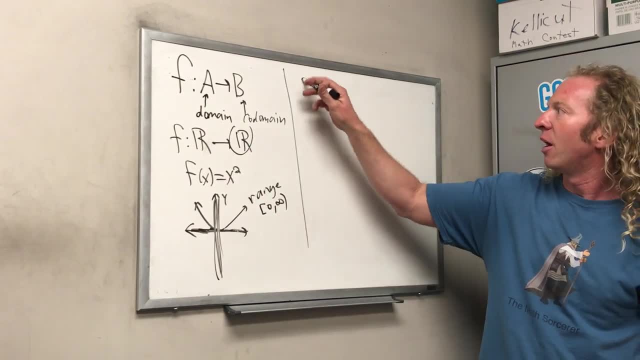 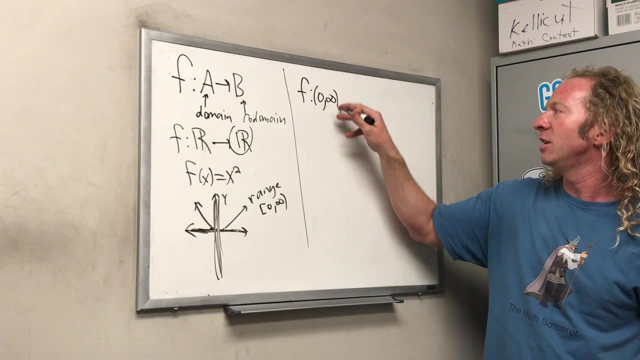 this case they're both the same. Here's another example. Say we have F from let's do some fancy notation, or not. How about just keeping it simple? Zero to infinity, to the set of real numbers, And this is a famous function. F of x equals the natural log of x, right The natural log. 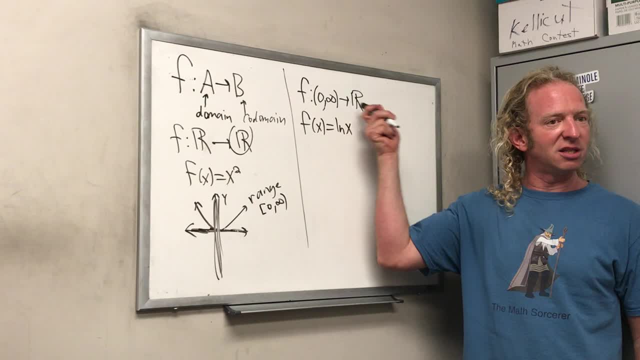 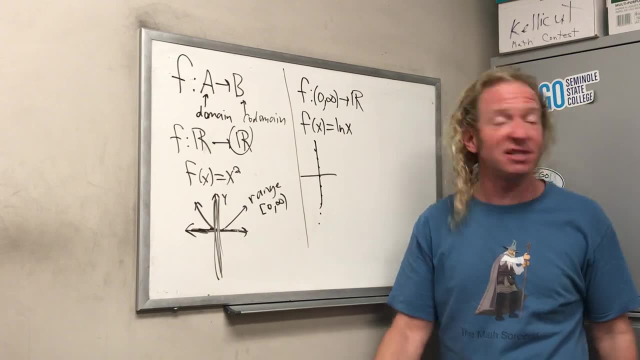 of x. So in this case, this is the domain and this is the codomain, right? In this case, Can we also write that as positive reals? That's exactly what it's going to do, Kyle. Yes, yes, I was going to write it like this. 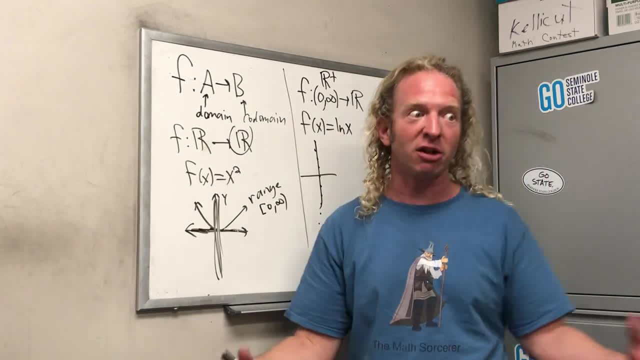 right, That's the set of positives. That's what I wanted to do. When I said fancy notation, I was like, oh, let me do that. But for some reason I became weak and didn't do it. So that's the graph of ln. 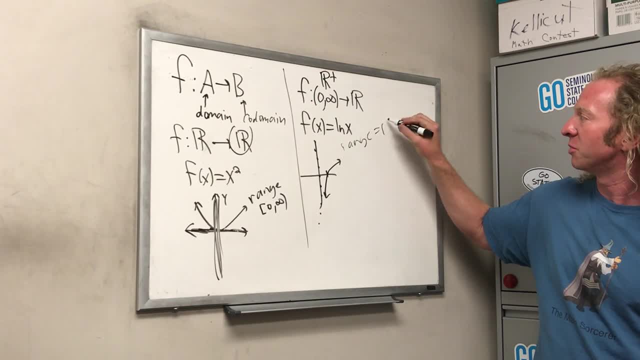 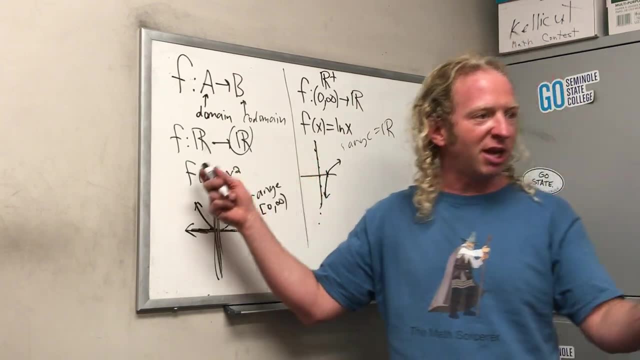 Oh, look the range. The range is equal to the codomain, right? So this is an onto function. Okay, so now that we have that out of the way, we have some terminology out of the way, So we have domain and codomain. All right, let's talk about injective functions. So, injective functions. 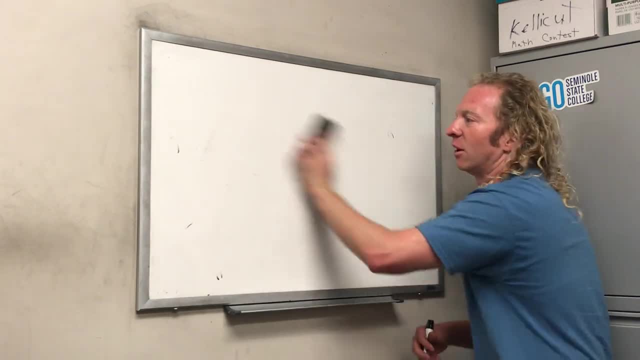 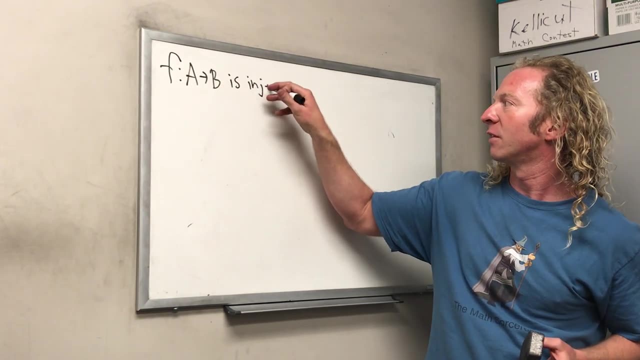 are super key. So we say a function F from A to B is injective, So injective It's also called one-to-one. So you can do this, So one-to-one. So you can do this, So one-to-one. 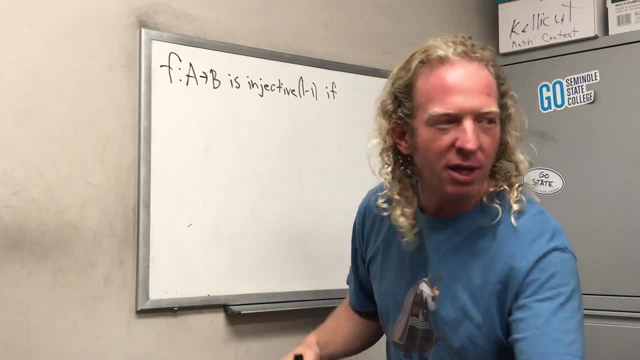 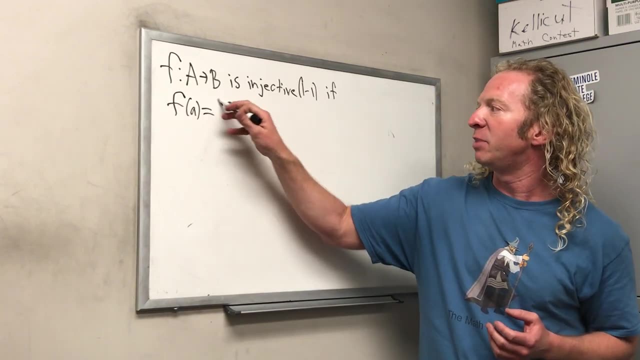 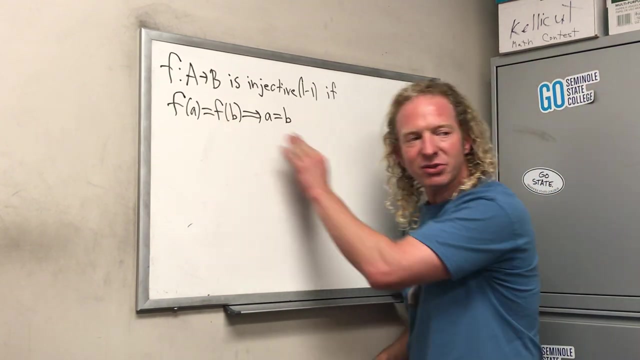 If, whenever the outputs are the same, the inputs are also the same. Okay, so equal outputs give rise to equal inputs. So if you have F of A equal to F of B, this implies that A is equal to B. So equal outputs give rise to equal inputs, right? 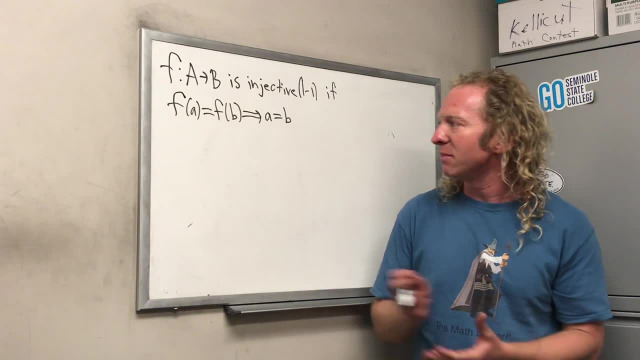 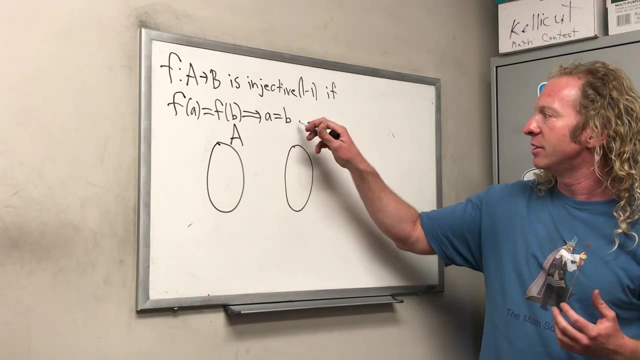 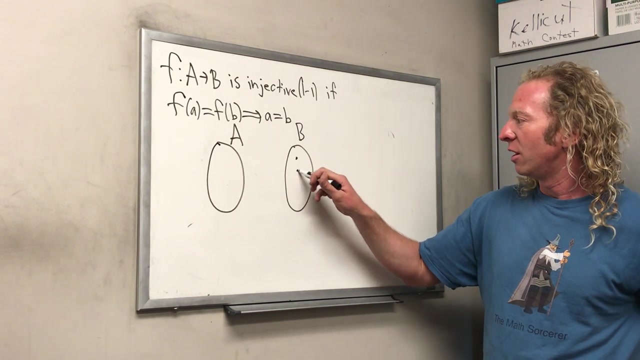 So what does that mean intuitively? So if this, if I can try to explain it, if this is B right, So what would be an example of an injective function? So there you go from one point to another point. Yeah, so like point maps, So like this point here would 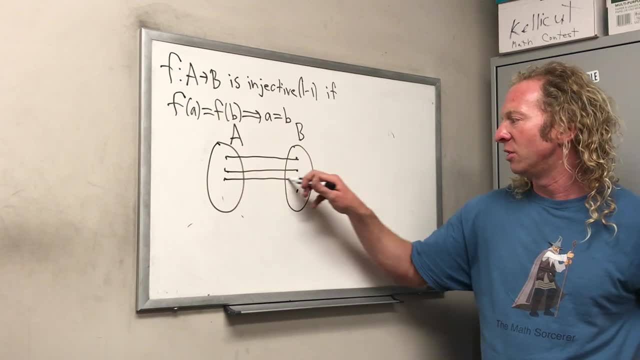 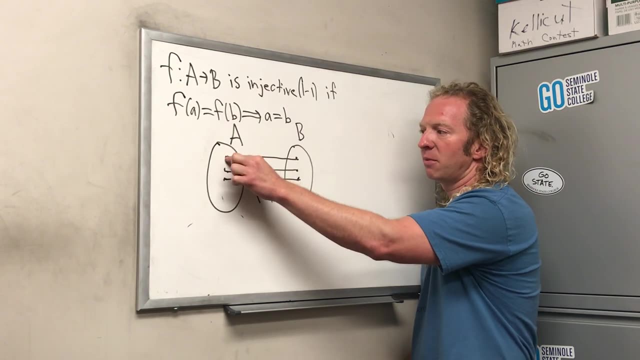 go here, This point here goes here And this point here goes here. That would be, that's injective, That's one-to-one right. So everything gets hit at most one time. So this number goes here, this number goes here, this number goes here. You can't have this. This is an 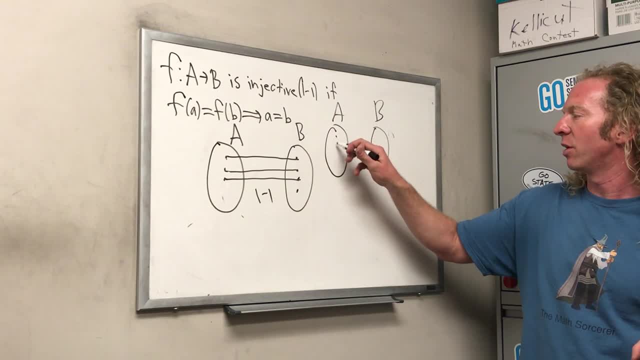 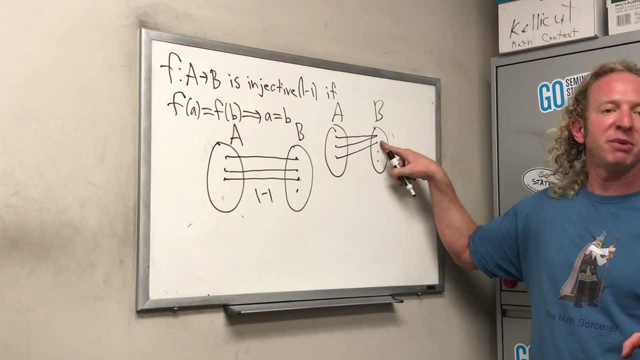 example of something that's not one-to-one. So here we go: one, two, three, One two, three, four. So this one goes here, this one goes here and this one goes here. This would not be one-to-one right, This would not be. 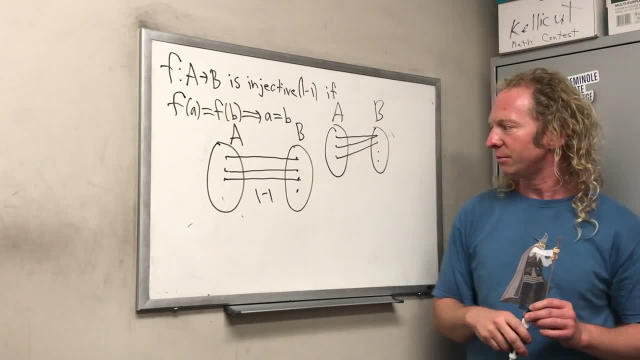 one-to-one. Your first example that's injective, but it's not surjective. It's not surjective Why? Because this one is not, It's not mapped, It's not mapped to. yeah, We'll talk about that later. So one-to-one intuitively means: 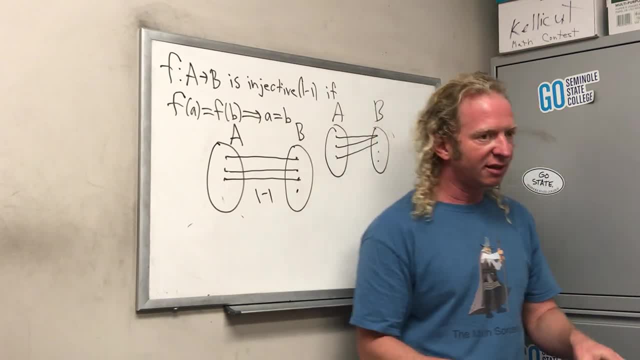 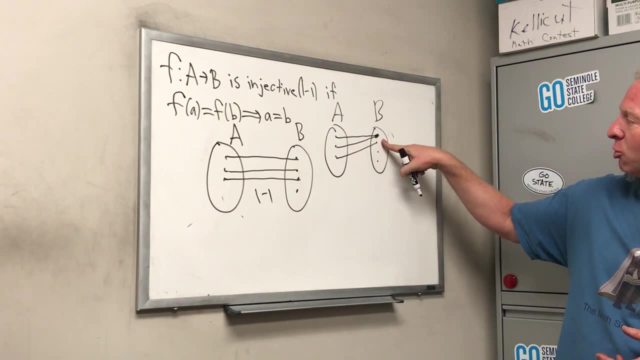 that everything in the codomain gets hit at most once. So this one does not one-to-one, because this y-value, this element, it's not one-to-one. This element in the codomain gets hit twice. That's what it means intuitively. That's what 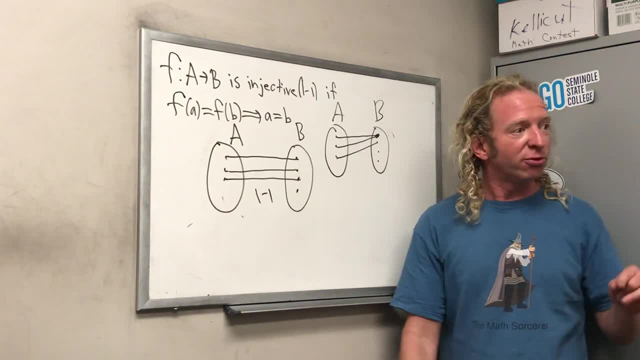 it means intuitively. That was kind of rough, but who cares? Let's do a proof. Let's prove a function is one-to-one. Let me show you how to do that. So I'm going to erase this and we'll prove a function. 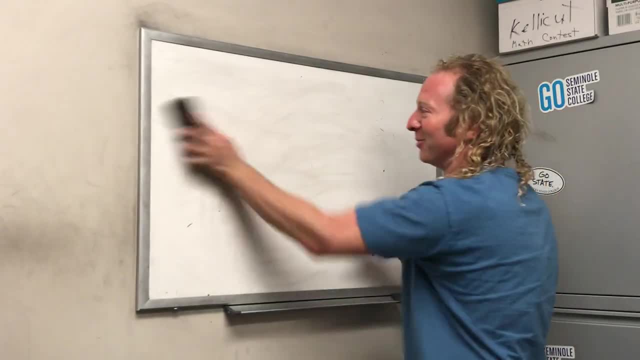 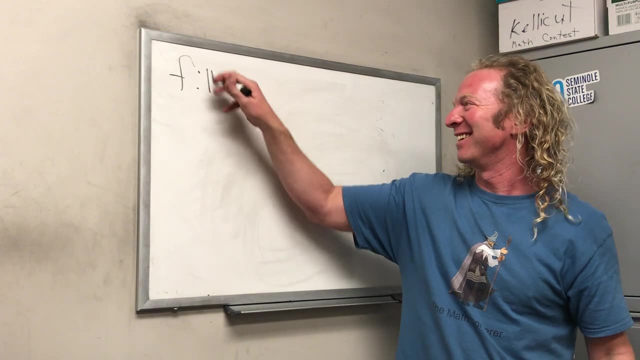 What happens to the eraser? Oh, it's over there. Well, no, I'm kidding, This is recorded, It's all right. No one knows where I am, so we take My name's Joey, All right, So we have a function. 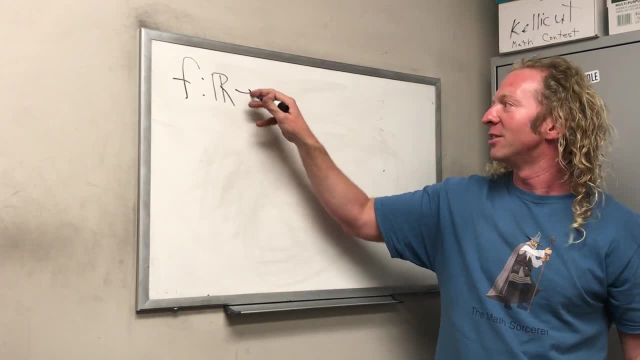 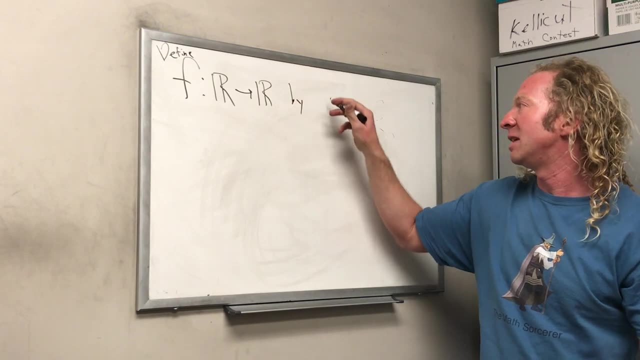 Let's do an easy one. So from the set of real numbers to the set of real numbers. So define this by I don't know. Let's keep it really simple. F of x- I don't know. It's late. 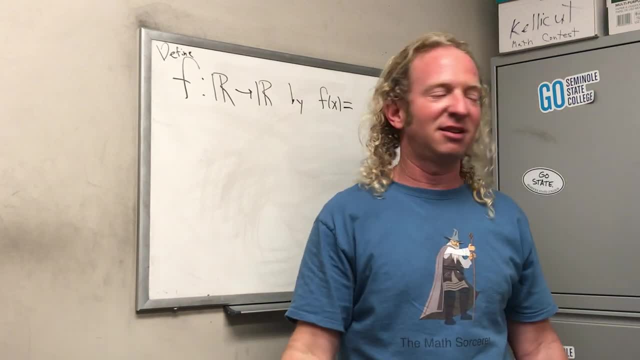 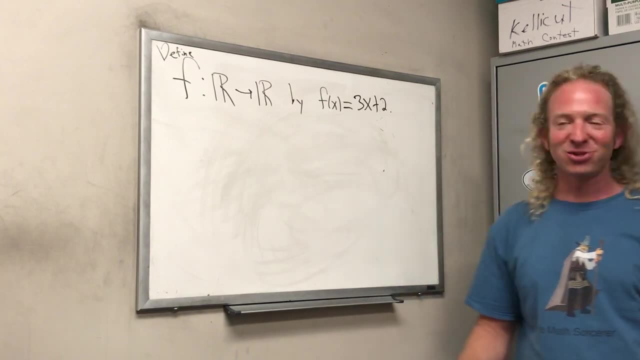 What time is it? 5?? 5 to 16?? Yeah, Let's keep it simple. Baby steps: 3x plus 2.. All right, Straight line. All right, Straight line. So we're going to prove it's injective or one-to-one. 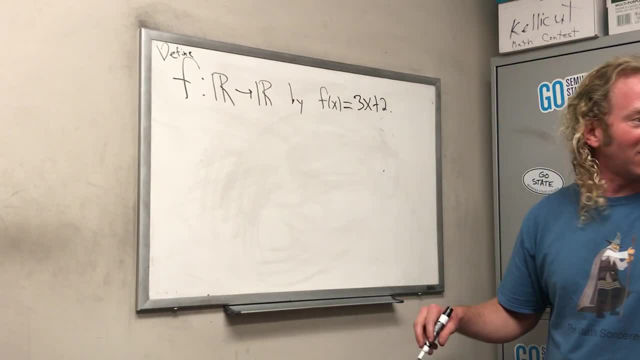 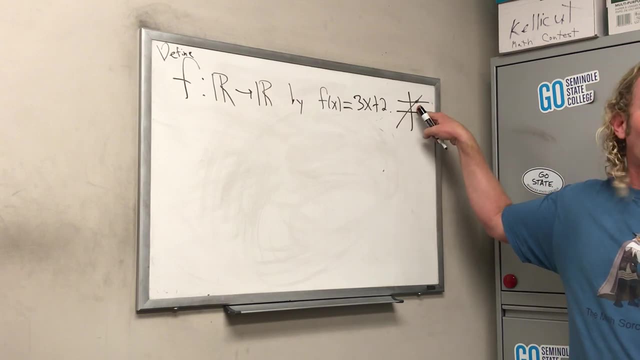 By the way, you know something from math: The horizontal line test. Remember that The horizontal line test Mm-hmm Right Crosses one time It's one-to-one by the horizontal line test, Right. So anyways, that's the same thing. 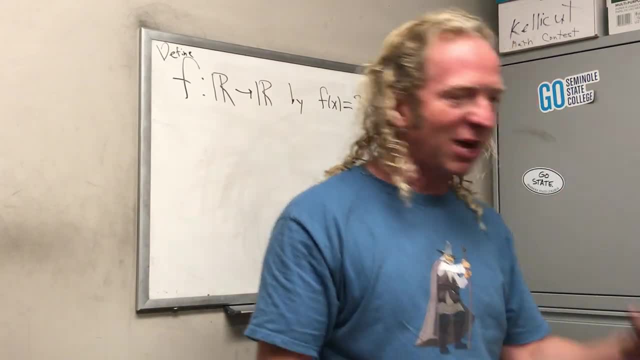 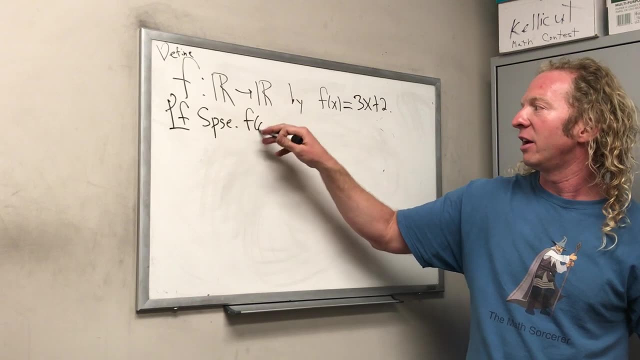 All right. So remember the definition said: whenever f of a is equal to f of b, we have to have a equal to b. So proof. So we start by saying: suppose that f of a is equal to f of b. You always start your one-to-one proofs like this: 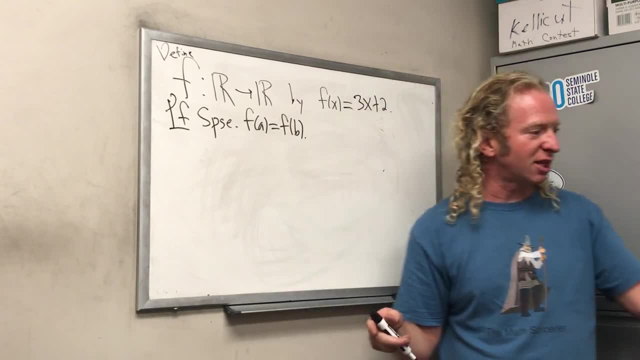 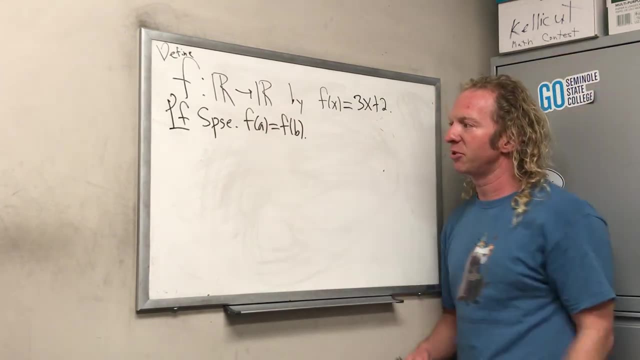 So if you take any kind of discrete math like, Aren't you doing CS? Maybe, Possibly, If you're doing discrete math, you do stuff like this. Right, It's part of a discrete math course. Oh, So suppose the outputs are the same. 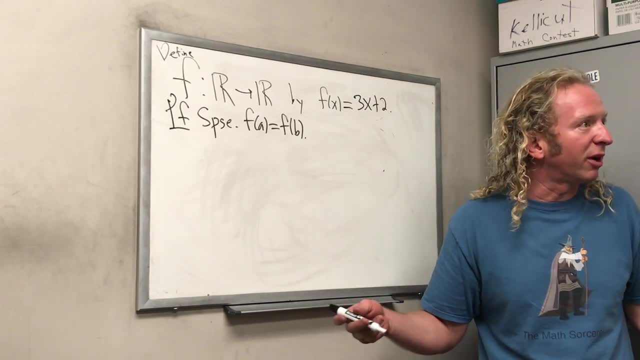 Now we have to show that a is equal to b. Well, there's only one thing to do at this point: Right f of a, you just plug in the a. So then, what would f of a be in this case? 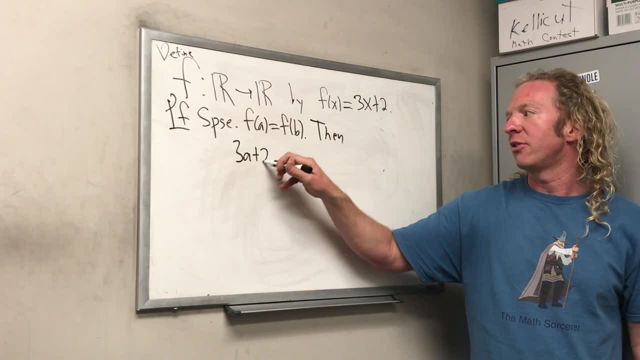 What do you think? 3a plus 2.. Very good, Yeah, 3a plus 2.. b plus 2 is now equal to 3b plus 2.. Boom, Like a pro. That's how pros do it. 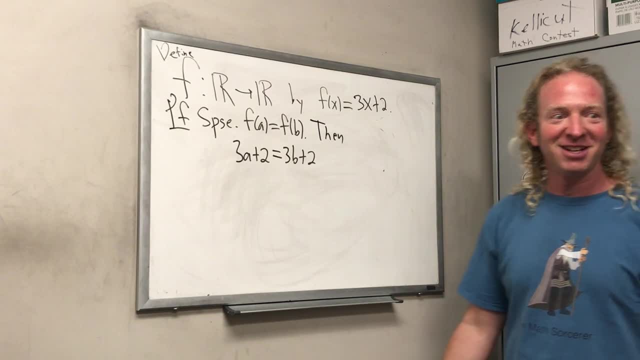 Right. So you're just plugging in the a, plugging in the b- Piece of cake, Right? Does that make sense, Cody? Sorry, Sorry Charlie, It's 3a plus 2.. 3a plus 2 plus 3.. 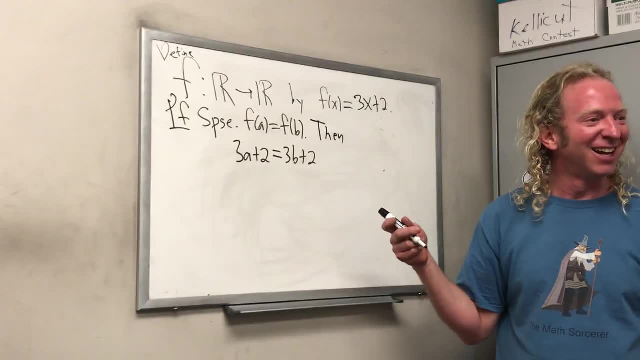 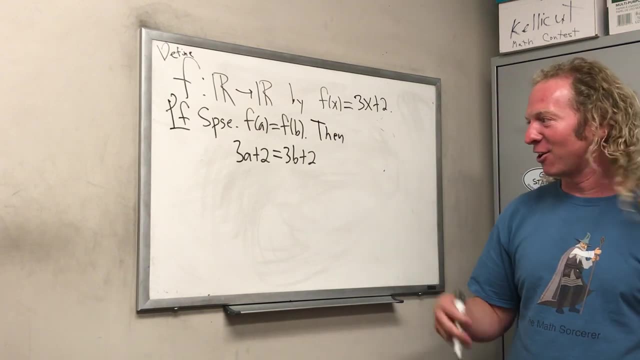 Shook, Huh, Shook. What is it Your? what? Shook, Shook, Shook. That's from a rap song Like that: Mobb Deep, Mobb, Deep, Shook, Scared to look, or something. 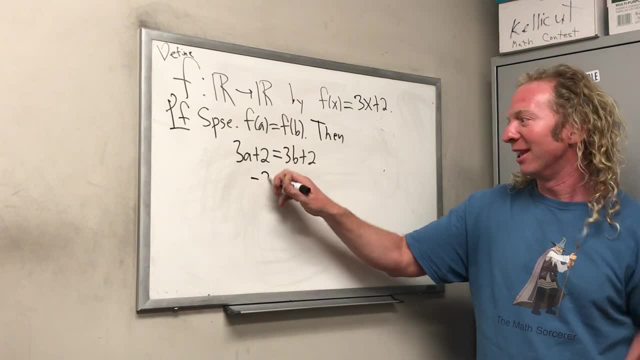 I don't know, So then I know the whole song, So we can talk about that later. So minus 2.. We should make rap videos. And then how do you solve this? What do you do now? Divide by 3.. 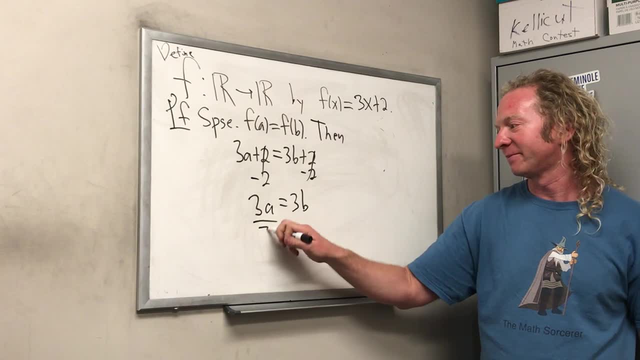 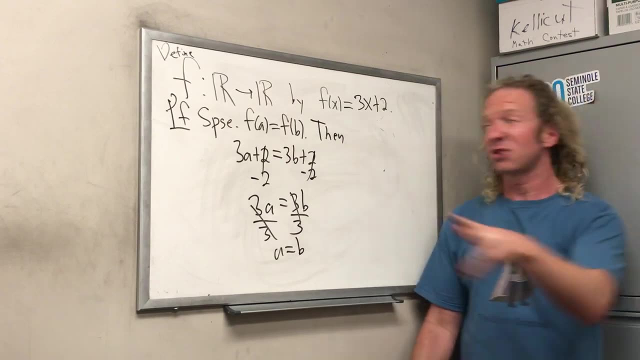 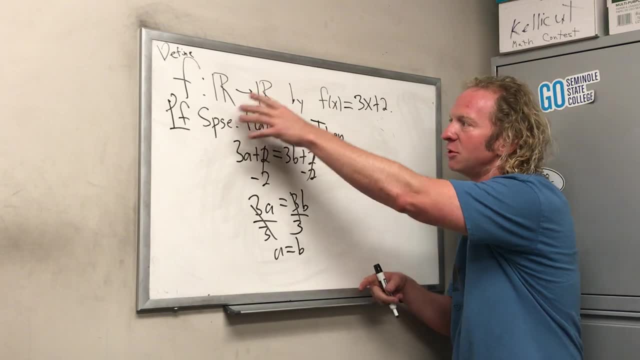 And also why we use the variables is because we need to show that it works for all values, Right. You remember hearing what Kyle said: That it works for all values, Right. Typically we would say: you know, for some a, b in the domain. 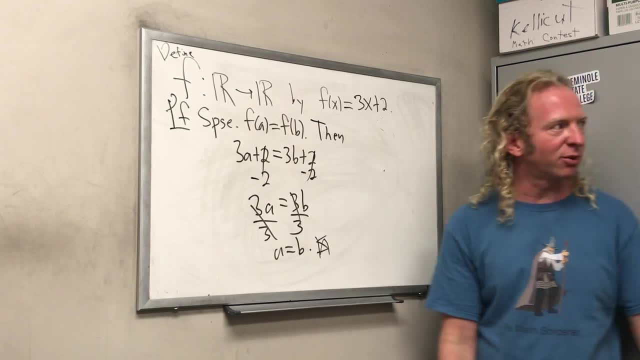 But I was being a little cursed. So that's it. This shows that it's add 1 to 1.. The proof is complete. So that's how you show a function is 1 to 1.. It's tough on this but it's because, like a lot of proof classes, that if you just 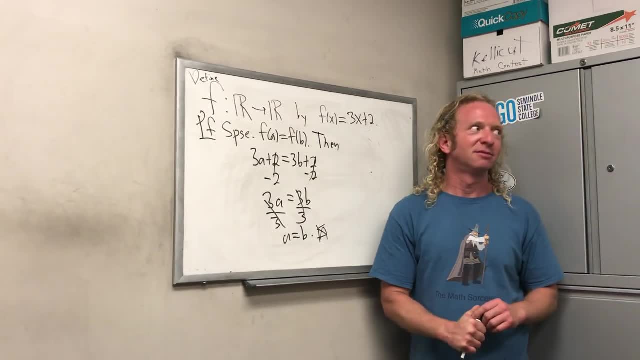 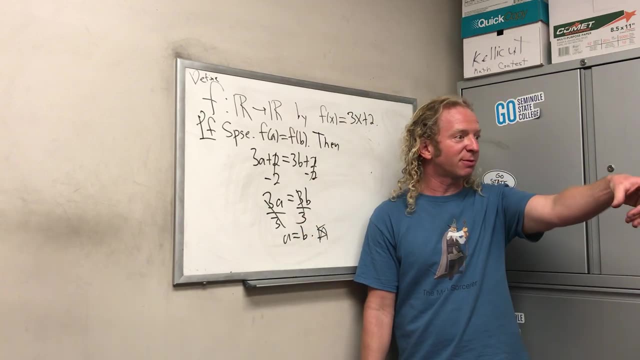 put in a number. you know, just say, put in a number, that's not good enough because it's just true for that value. the linear algebra stuff with the matrices, A lot of people would turn in, they would write numbers. I just, I didn't even look, I just crossed it out. 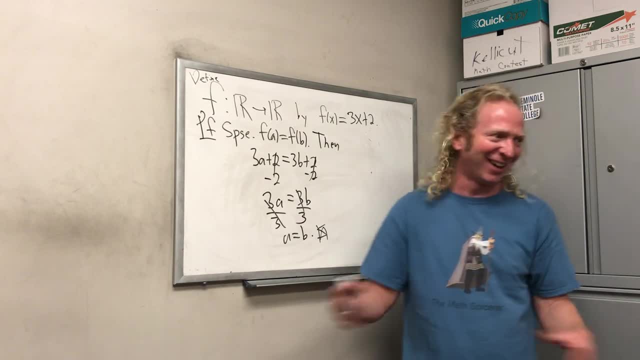 I didn't even give it back. What plug in numbers? No, Yeah, what? Yeah, yeah, because you have to. yeah, yeah, I don't even that's the most common thing- Like it's like yeah, people are like. 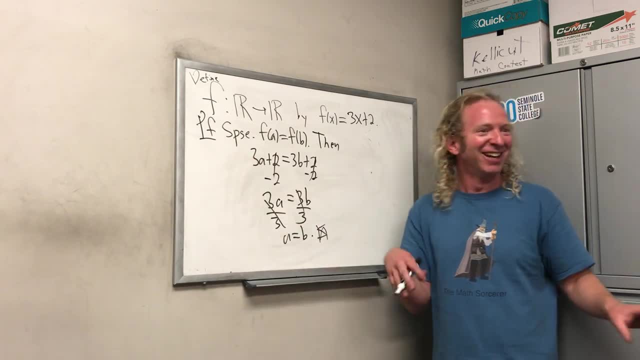 oh, three by three matrix. what's the matrix? Well, we make one up Like you can't do that, right? All right, so that's one-to-one. So, basically, you do this and then you show: that's true. 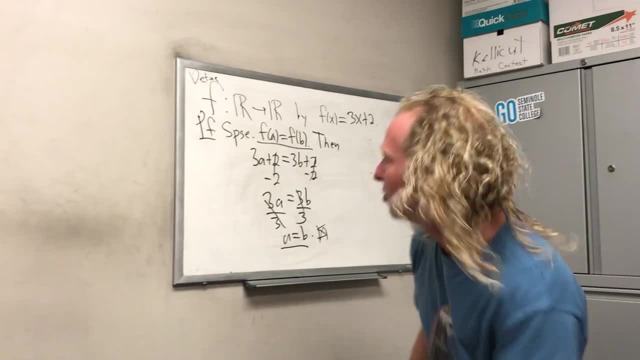 and that's how you show it's one-to-one Make sense. Yeah, All right, let's do one-two now. Let's do one-two really quickly. Ooh, maybe I'll show you something cool at the end. Ooh, I have an idea. 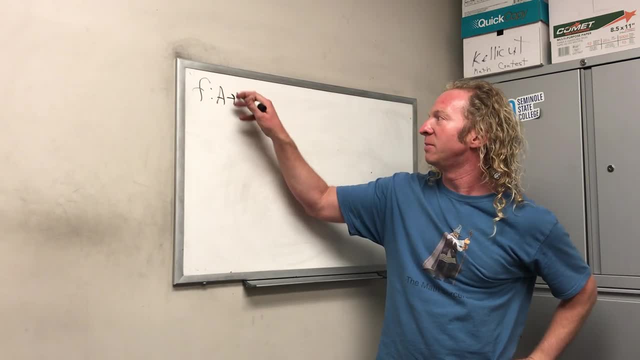 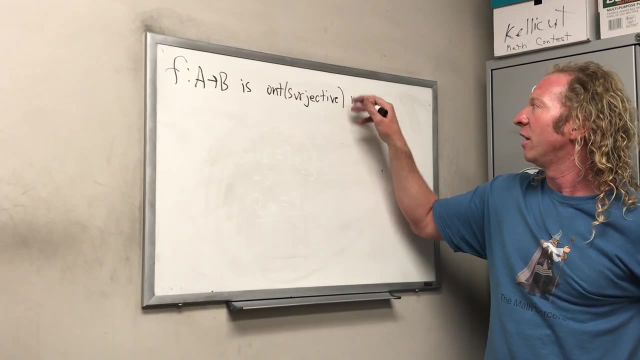 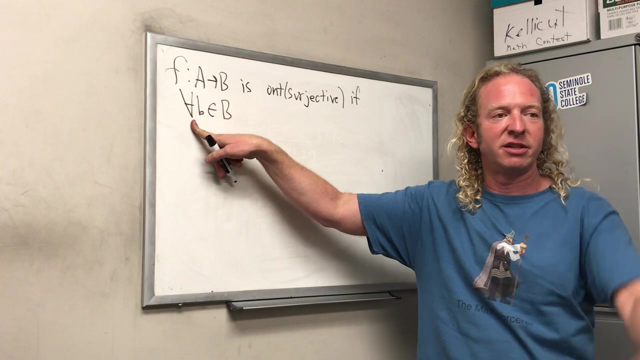 Oh, maybe, maybe, Okay. so let's define onto really quick. So F A to B is onto or surjective. if so, for all little b in capital B, that means for all in math. So I don't know if you've ever seen that, Dylan. 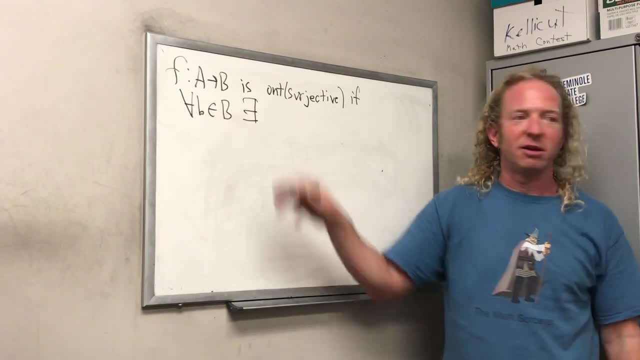 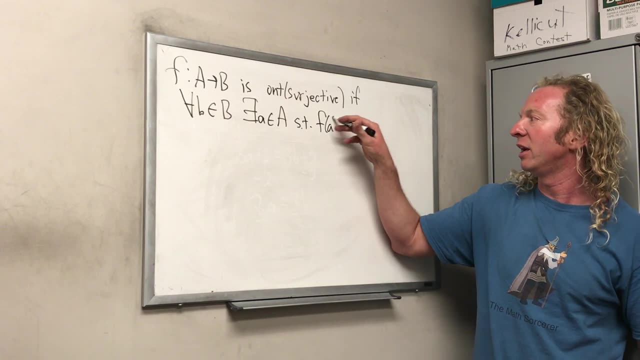 For all little b in capital B. What's this backwards E mean? It exists, There exists. there exists a little a in capital A, Such that F of little a goes to little b. This is beautiful, And again, ooh, it says onto: 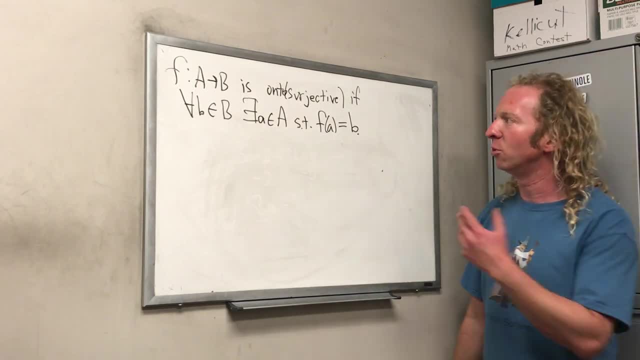 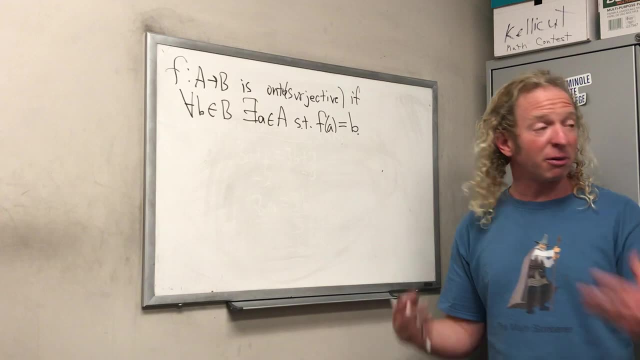 I can't emphasize how important this is for math. I mean most people who learn this stuff, like most people who like go on YouTube and search for this stuff. they're probably like in a discreet math class, But in higher level math, like when you study accountability. 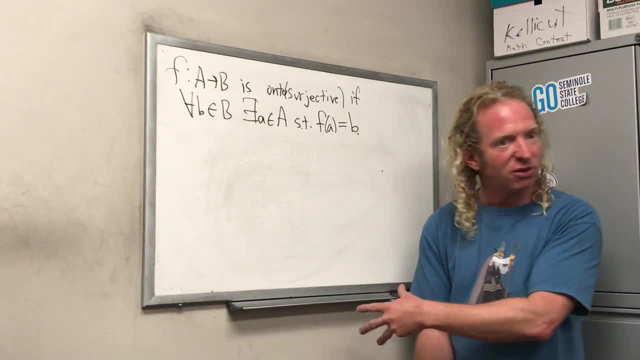 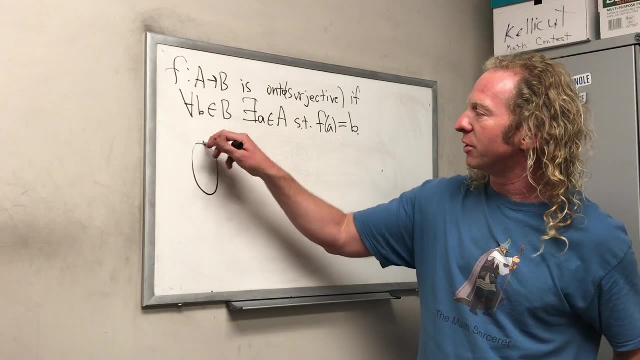 like showing two sets have the same number of elements. it's called cardinality. It's the same thing, right? Anytime you're showing, anything is the same, and isomorphism, stuff like that. you have to know this stuff. So, basically, what does this mean intuitively? 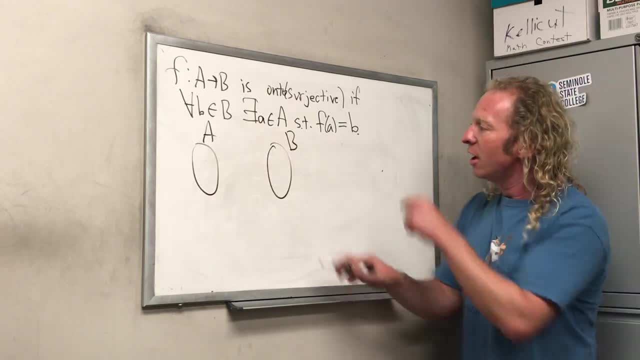 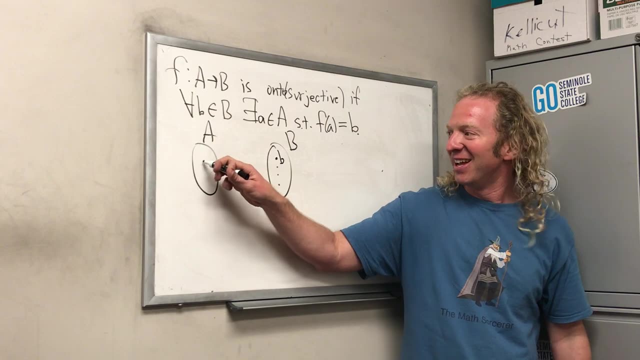 So here's A And then here's B. So it means for any little b here that you pick, you can pick any of these. No one gets left behind. You can find what's that? No one gets left behind. No one gets left behind. 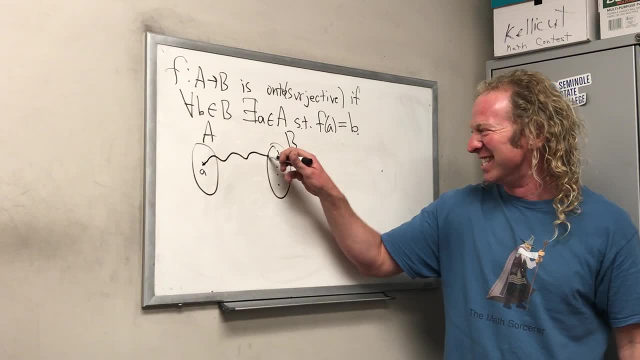 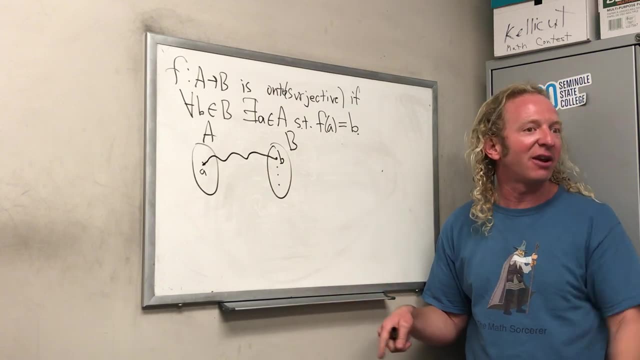 That's right. That's a great definition. Yes, yes, yes, So you can find a little a that goes all the way, all the way to B, right. So everything gets hit at least once. all right, Everything gets hit at least once, right. 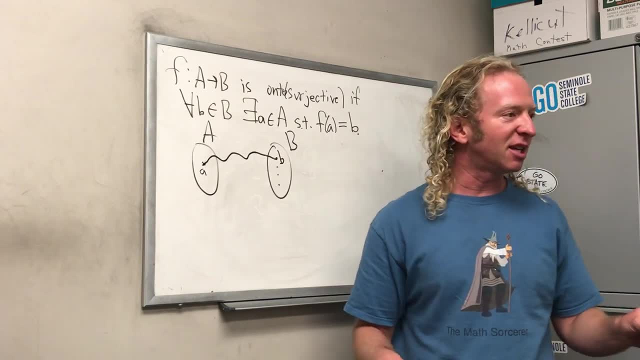 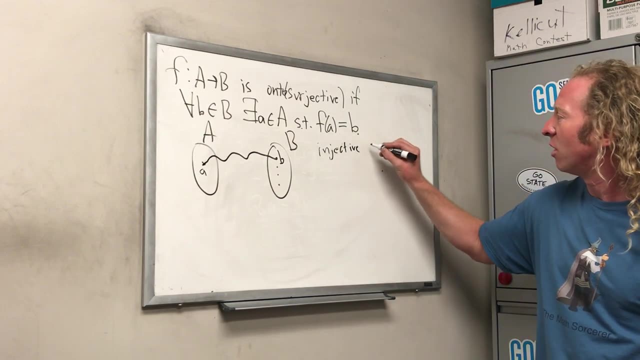 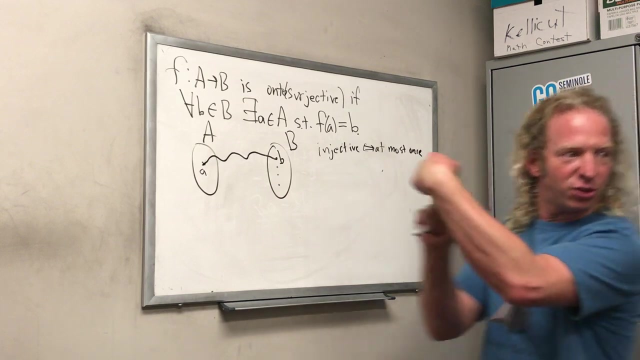 So injective meant everything gets hit at least once, At most once, right, So just so, injective was at most once, So nothing can get hit twice. remember that With the injective we had the two, the two things. 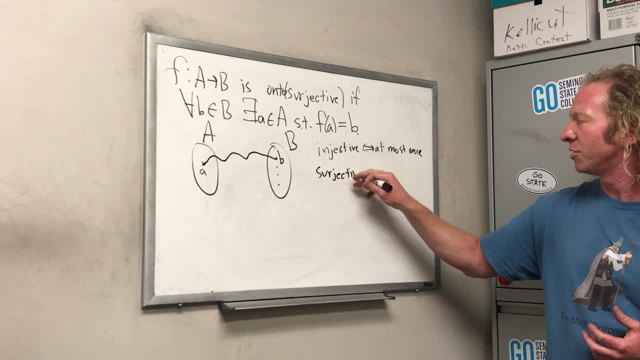 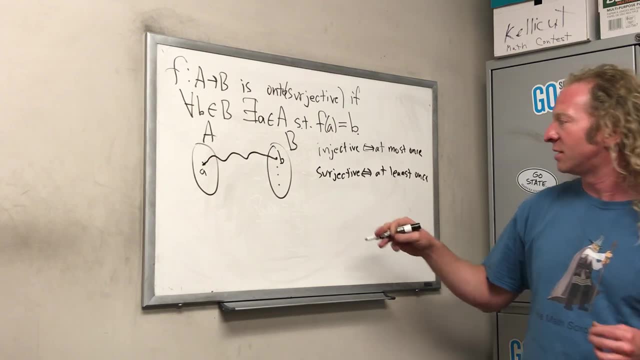 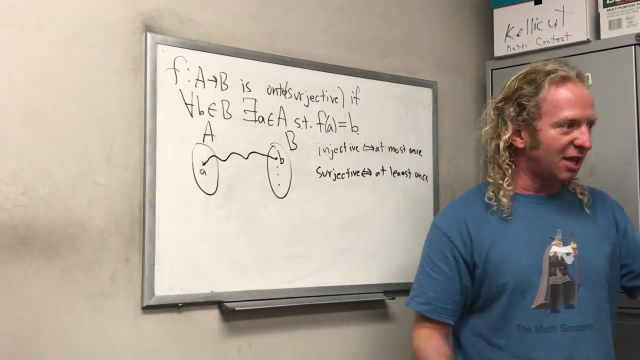 And we're saying surjective, surjective, we're saying it's at least once. So if everything gets hit at least once and at most once, so both happen. Can anyone put that into words? Subjective: Yeah, so if it's at least once and at most once. 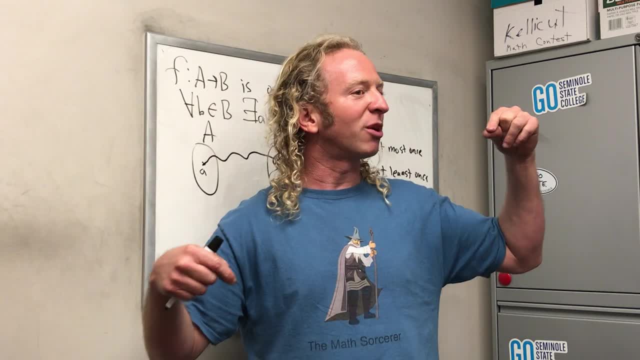 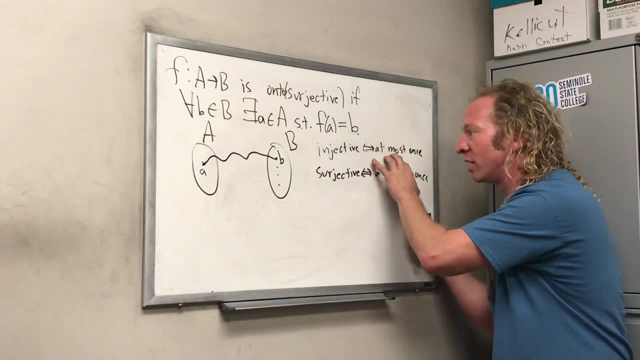 what's another way to say that Everything gets hit? what am I looking for? Anyone know? Eggs, eggs, eggs, Eggs. Exactly once, right? If everything gets hit at most one time, right? So check it out, check it out. 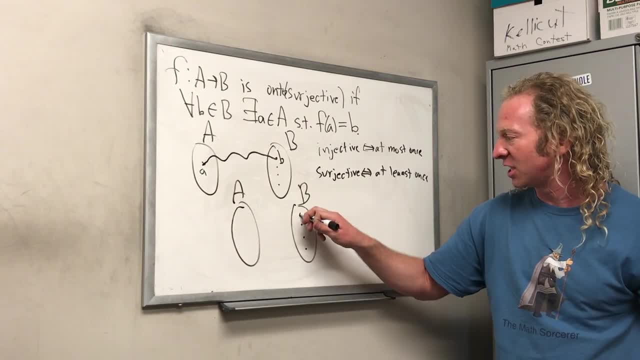 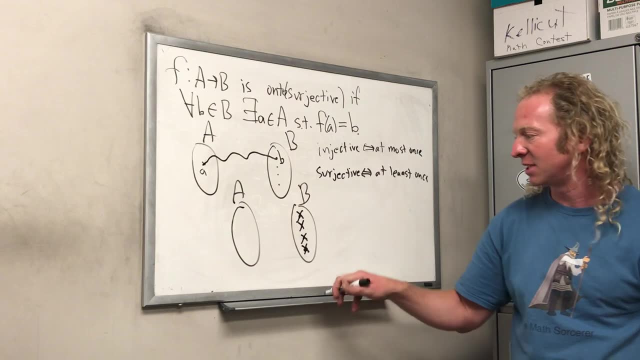 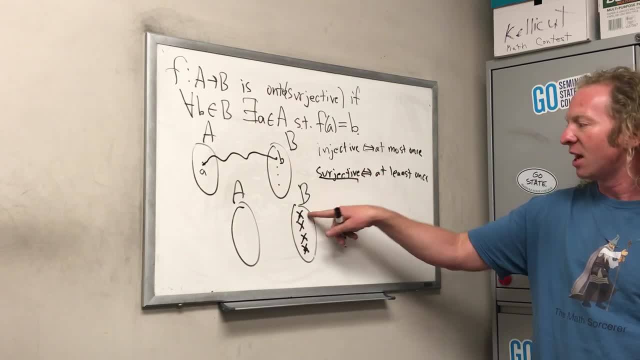 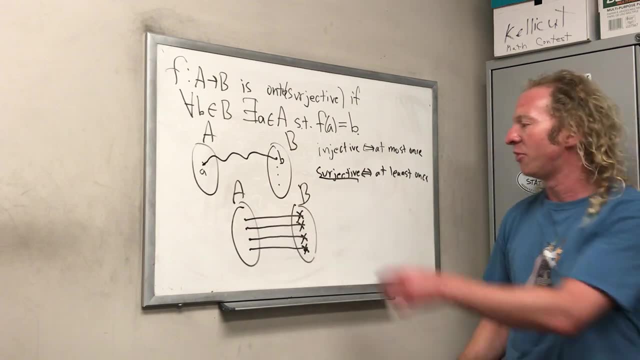 So everything got hit at most once, at least one time by surjectivity, At least one time by surjectivity, And then by injectivity. everything got hit at most one time. So then everything gets hit once and exactly once. When you put these together you get the word bijective. 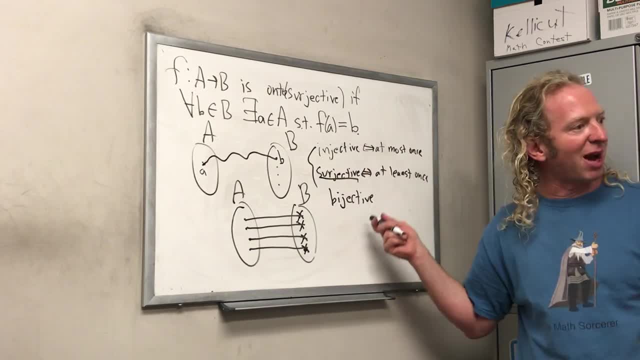 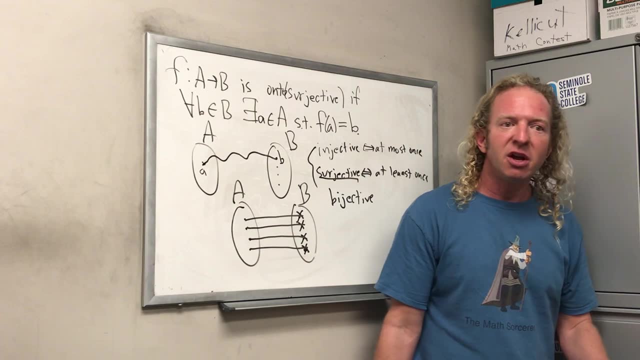 So if you have a function that is injective and surjective, it's called bijective or a bijection. Sometimes, like Lisa used the word earlier today- I don't know if you were here- she said one-to-one correspondence. When you use the word one-to-one correspondence, 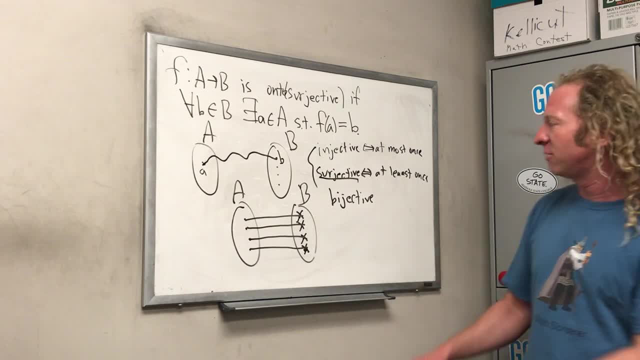 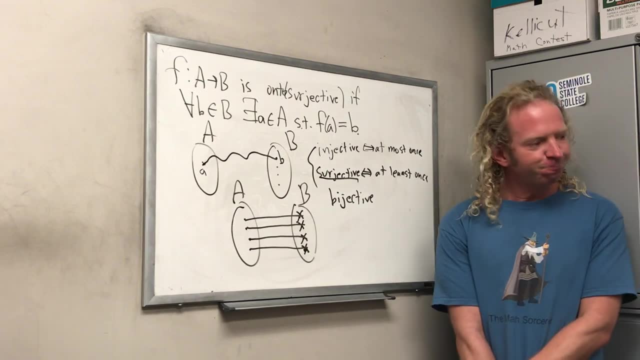 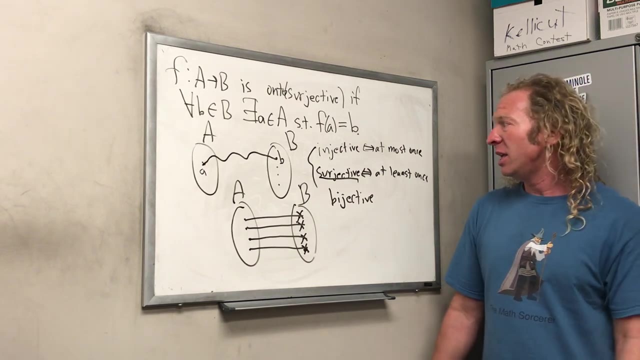 it's the same thing as bijective. So bijective means everything gets hit exactly exactly once, right So? yes, So when we're just playing with functions on regular pre-calculus classes, we're just only talking about bijective When you say a function's one-to-one. 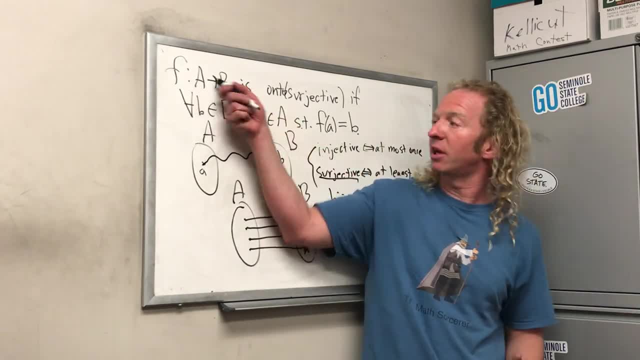 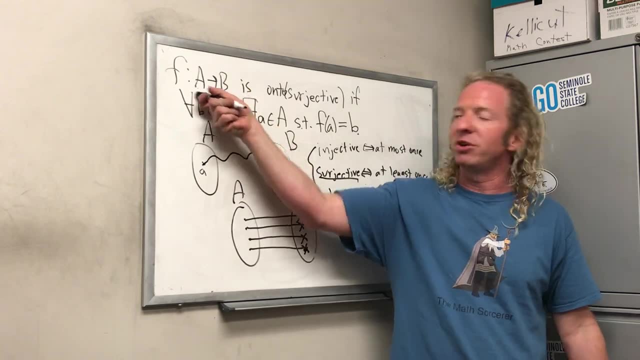 Yeah, yeah. they don't even talk about surjective, They don't even define them this way in calculus one, two, three courses. They don't need to. It's only when you get to like discrete math, computer science, advanced math, where you do this. 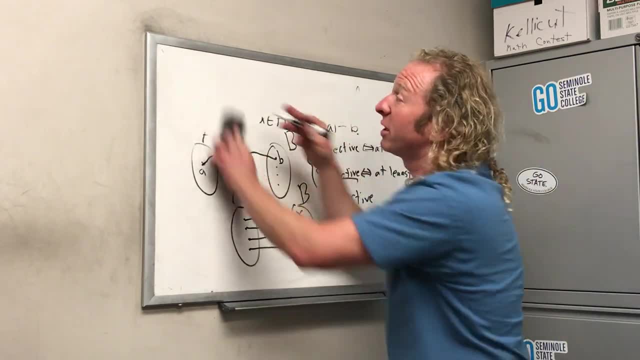 and then you start talking about stuff like this, And typically, Albert, they just do stuff like this right. They just say: f of x equals square root of x plus two. They don't give you the domain. They don't give you the domain. 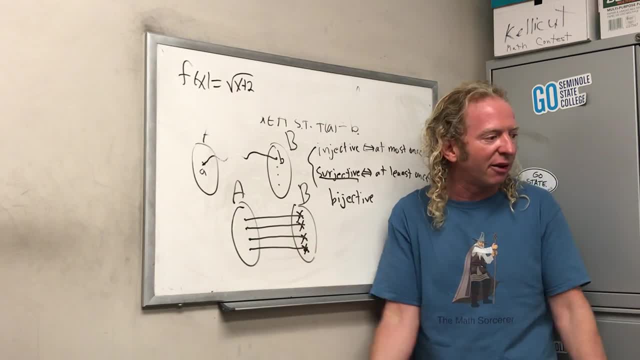 They don't give you the co-domain right. You just kind of like it's kind of implied You gotta figure it out. In high-level math, like in research papers and stuff, it's usually always just given Like. it's always, like you know, clearly defined. 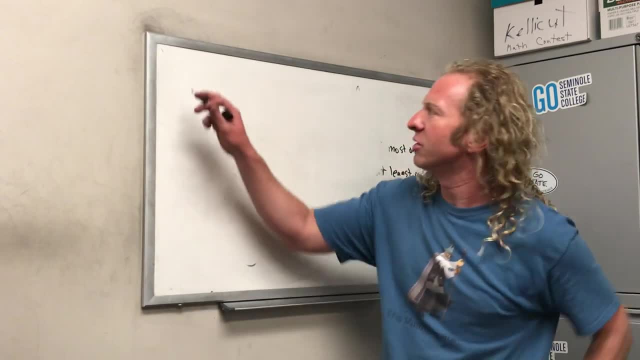 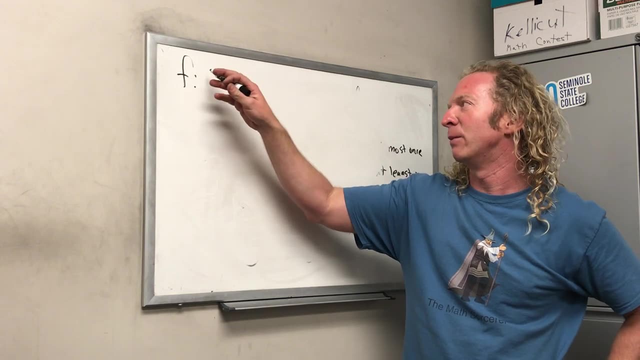 Let's do a simple example of showing something is onto. Let's try this one, So f. let's see if I can think of a better one. I can't think of a better one. I'm weak, I can't think of a better one. I can't think of a better one. 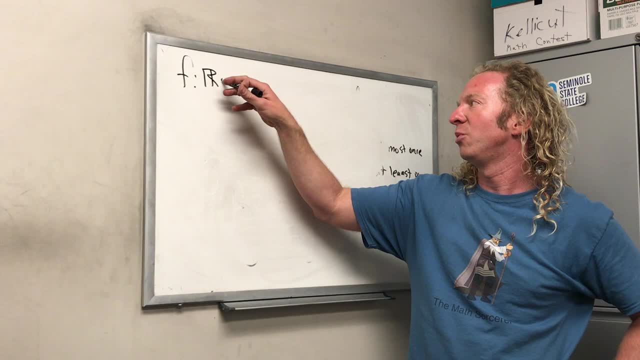 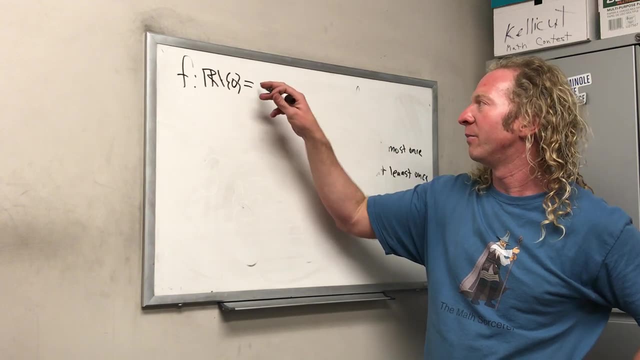 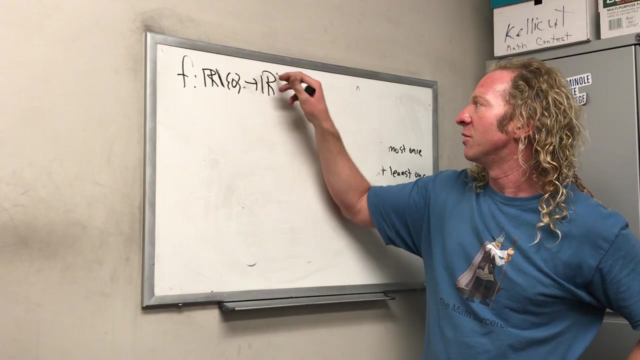 The real numbers. to the real numbers, set minus zero. to the real numbers: to the real numbers. Sorry, I'm thinking, I'm trying to come up with an example at the same time. So to the real numbers, set minus zero. I'm just using different notation to make you think. 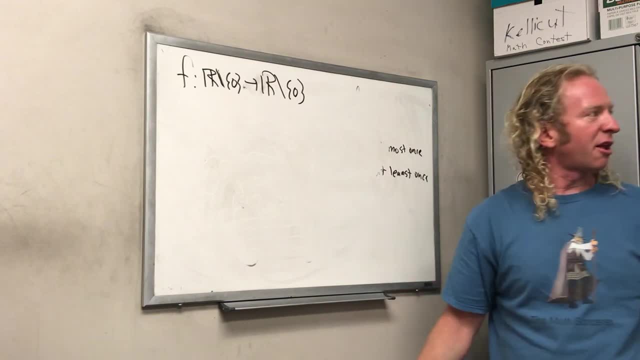 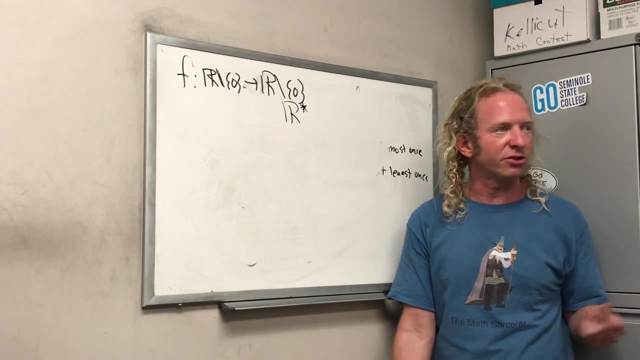 This means r set minus zero. This is all the non-zero real numbers. Another way to write this- I was thinking of Kyle, because he mentioned this earlier- is r star. r star is typically the non-zero real numbers. So if you see an r star, 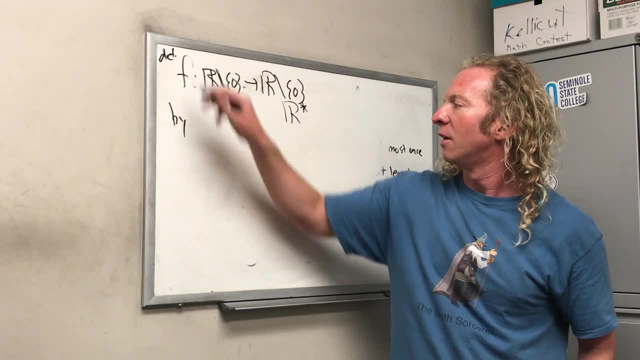 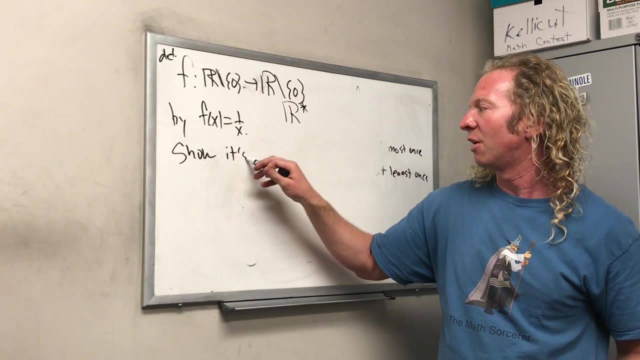 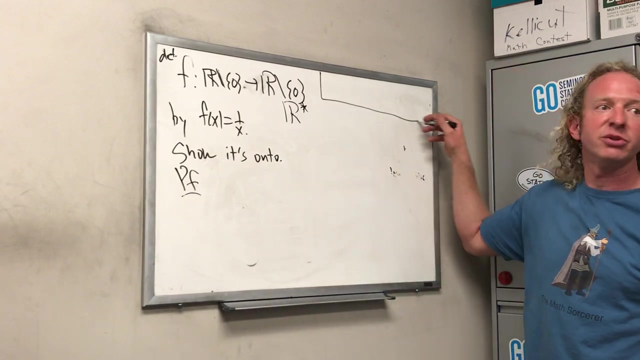 And let's define this by: so define by: f of x equals 1 over x. Let's show it's onto. show it's onto So proof. So just let me write the definition of onto up here again, so you see it. 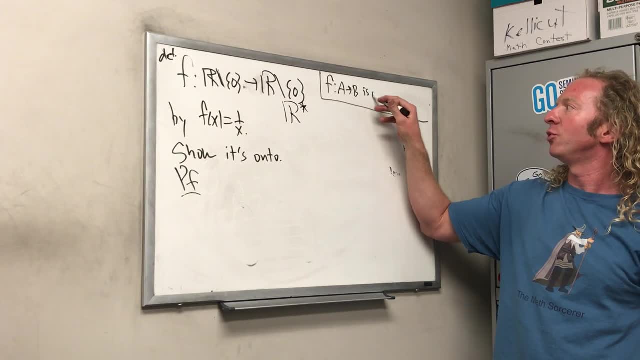 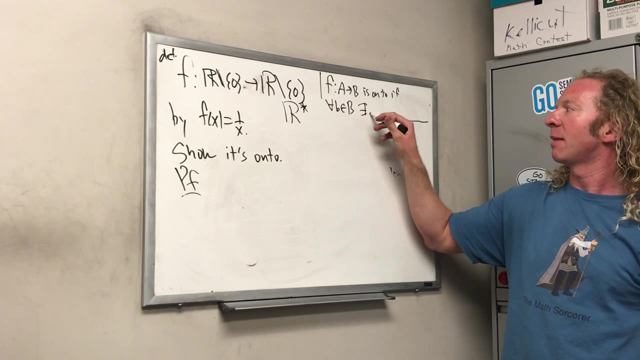 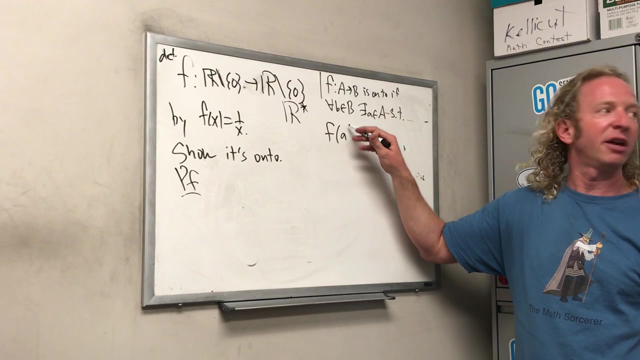 It's very key. So f from a to b is onto. if For all little b in capital B there exists a little a in capital A, such that anyone remember the rest, F of little a goes to b. Yeah, to b. 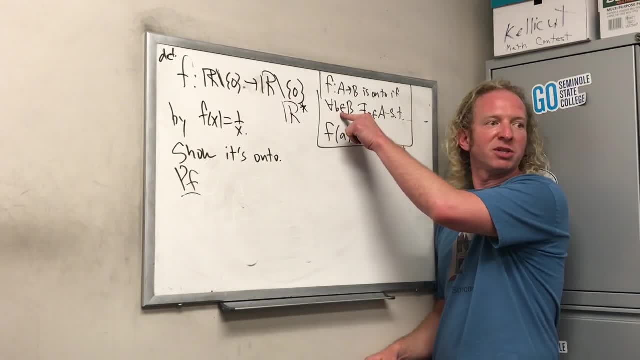 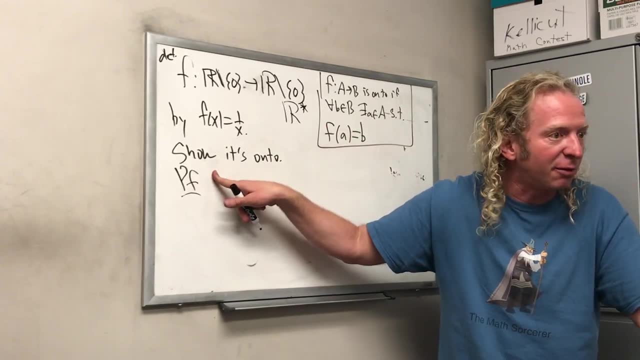 So that's the definition. So when you're satisfying this definition you always start with this condition here. okay, So you start by saying: suppose little b is in capital B, or take any little b in capital B. You can say: suppose it's arbitrary, and stuff like that. 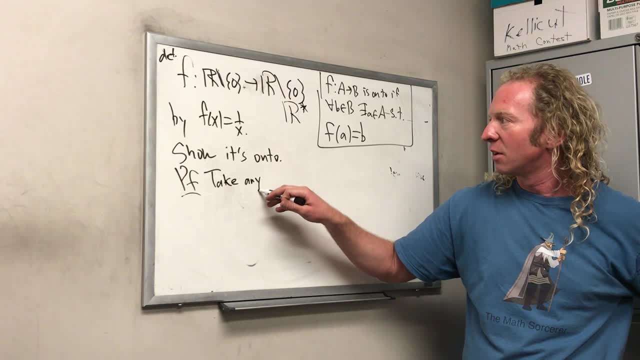 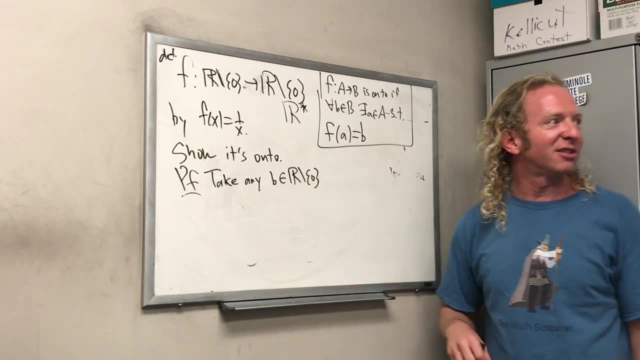 but I'll just be a little bit tercier. Take any b in this set here. I almost said group too much group theory. So take any little b in this little set here. right, One second, don't pause it. 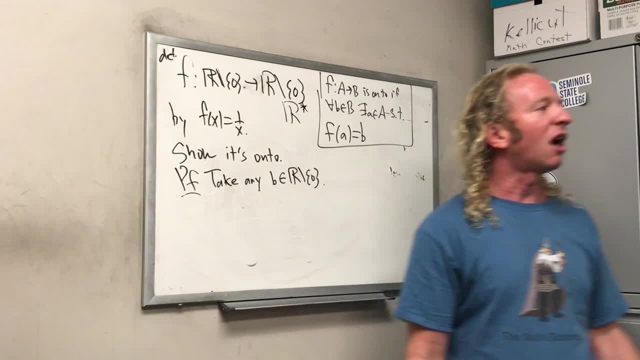 Hey, it's okay, I sent you an email. you're good, I can't get into my email. Oh, okay, you're good, though You're good until Thursday or Wednesday. you're good, I'll talk to you in like 10 minutes. 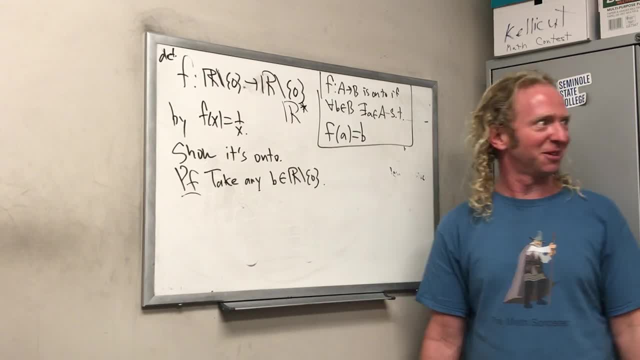 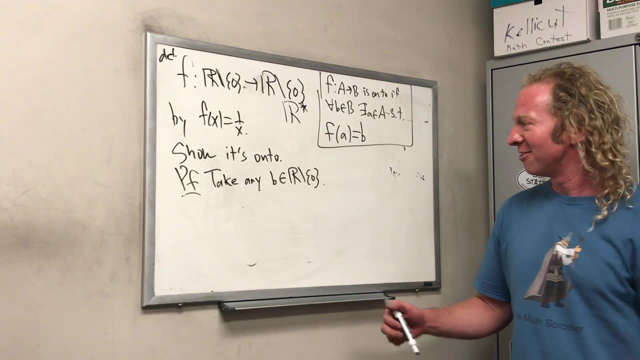 But you're good, Can you text me? I don't have a phone. I don't have a phone. Oh, you can't get into your email. Hang out for 10 minutes. you got 10 minutes. Yeah, hang out, stay here, stay here. stay here, hang out. 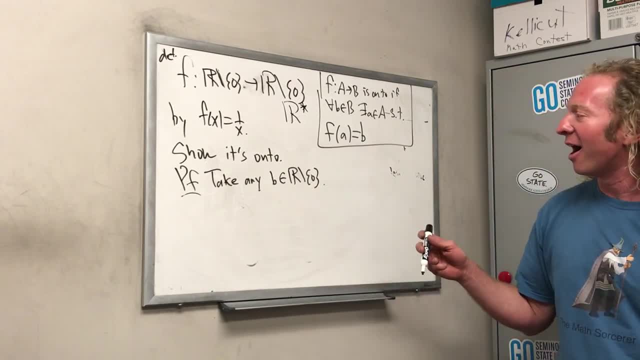 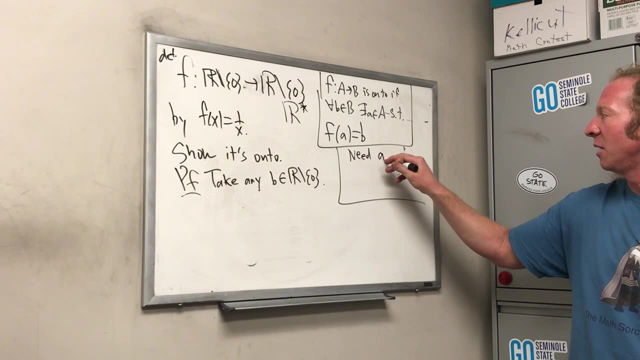 Kelly, take any little b here And then, so we have that. So we need what do we need? We need a such that we need this, right. That's what we need, right? You had it out, Yeah. 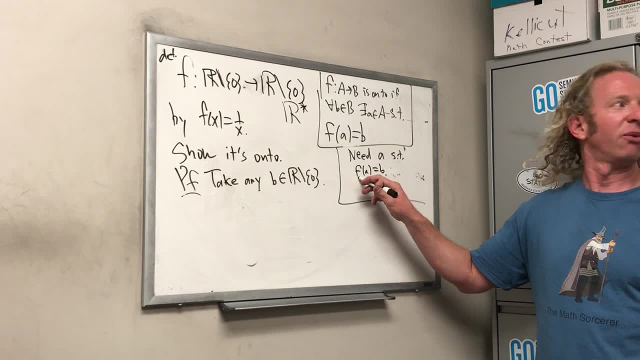 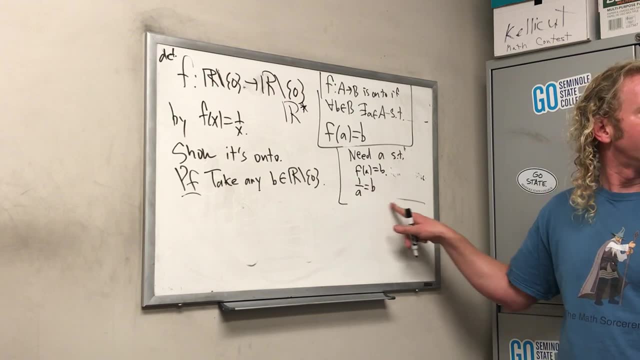 So what's f of a? in this case? 1 over x, 1 over a, 1 over x. So we need this Right. So we're working backwards. This is really key. Can you see, Kyle, Kyle. 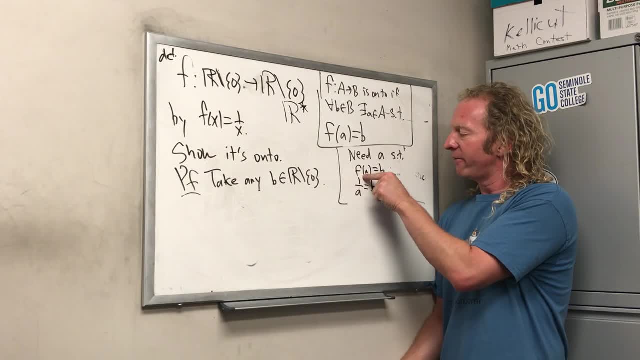 Can you see? Yeah, Yeah, So we need a such that this is true. So we need an a such that f of a is equal to b. So we're working backwards. This is how you figure the problem out. This is the most important part. 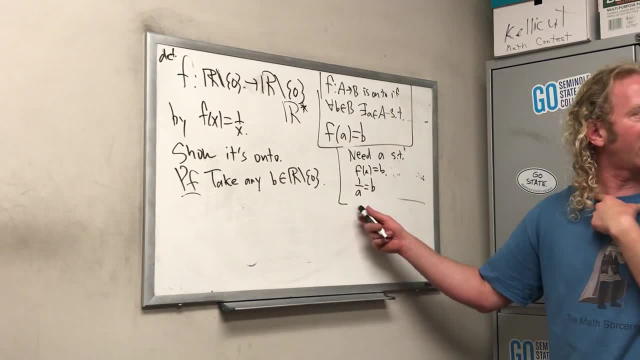 So f of a is 1 over a. So we have to solve this for a. How do we solve this for a? What do we do? What do we multiply by A, By a. So you put an a here. You put an a here. 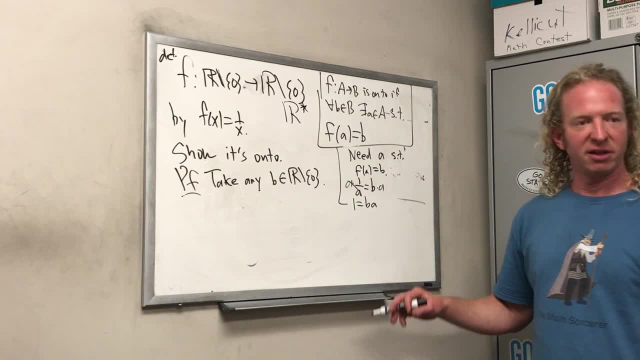 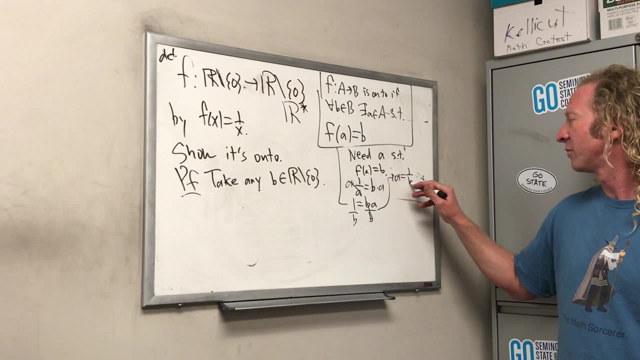 So you get 1 equals b, a, And what's the next thing you do? to solve for a? Divide by b, Divide by b, And so we end up with a equals 1 over b, Right OK? So now that's going to be our a. 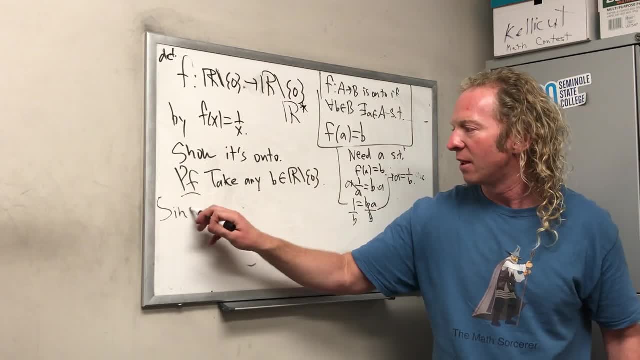 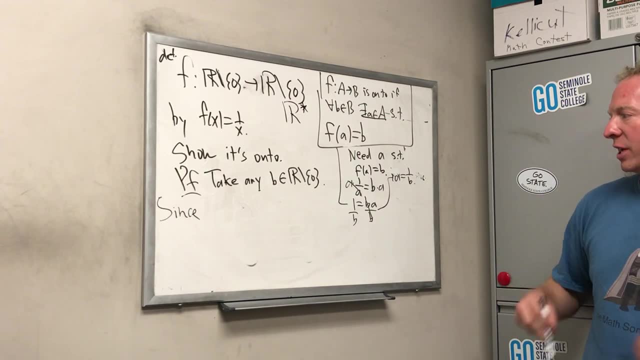 So then we take b in here. So then, since, OK, so this is going to be the a we want, Right, So we need to show it exists, OK, So in order to show that it exists, you have to explain why it makes sense. 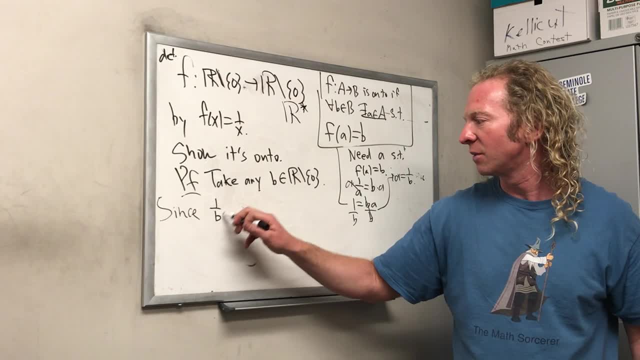 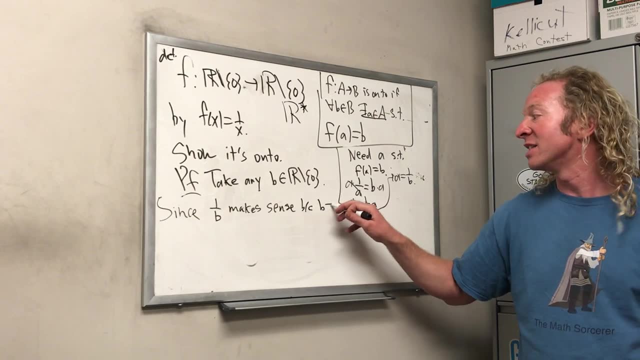 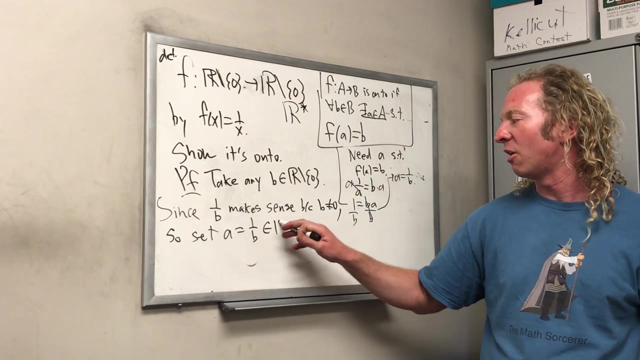 So note, 1 over b makes sense because b is not 0. So set a equal to 1 over b, which is in our domain. It's a little confusing because this is the codomain, This is the domain, Codomain domain. 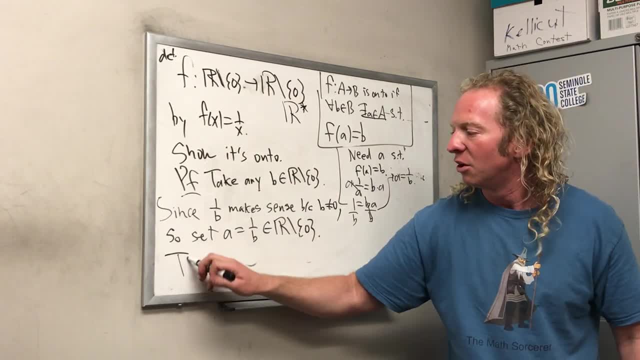 Codomain domain. Codomain domain- Right. Then we have to show that f of a is equal to b. So let's do it. So f of a, Right, So f of a. Well, that's 1 over a. 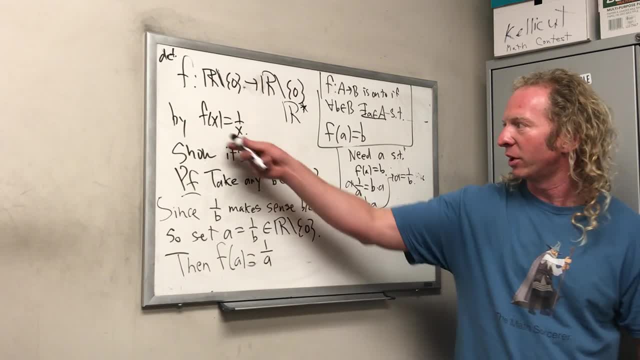 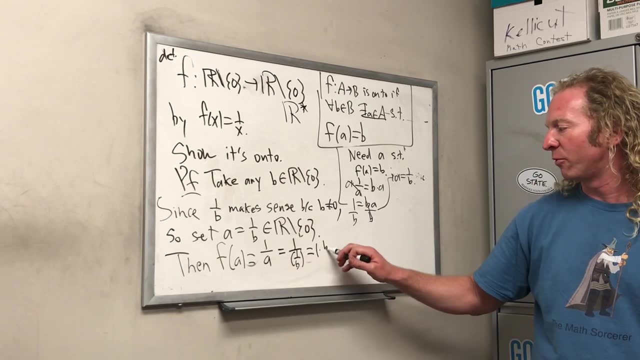 Plug it in here. And a is 1 over b, So this is 1 over 1 over b, which is 1 times b over 1, which is b. So look at that, We took any little b, Right. 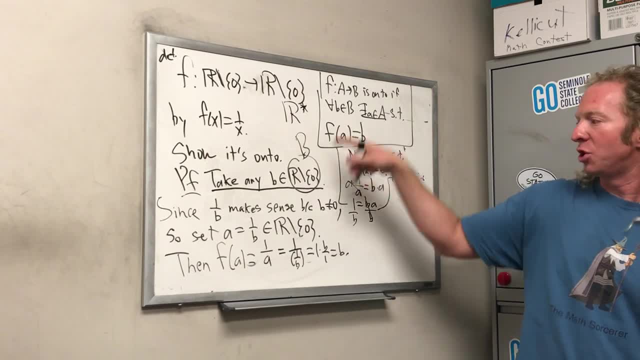 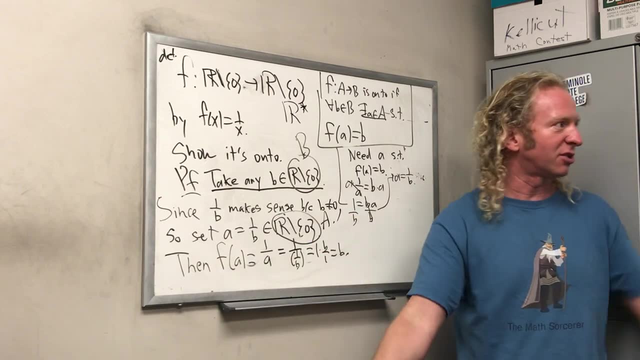 This is our big B. We took any little b in big B. We showed there exists an a in big a. This is our big a, such that f of a is equal to little b. That shows the function is a subjection. Yeah, 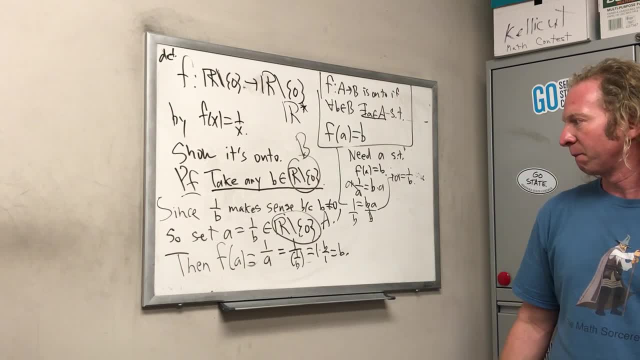 Would it be valid to say that also, since b is a positive integer? No, We have to specify that can't be equal to 0. It's not. No, There are real numbers here, So it doesn't have to be an integer in this case. 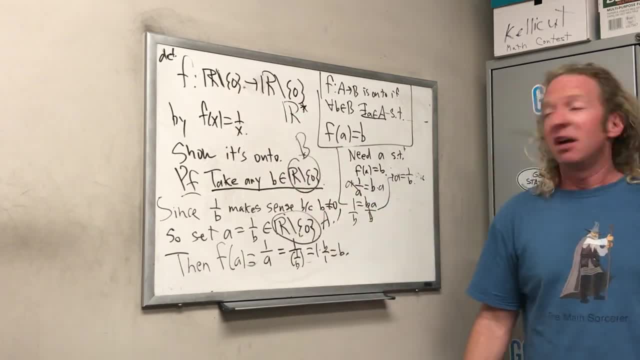 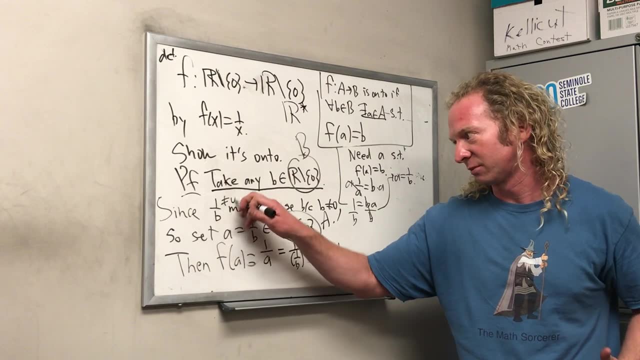 Right, Oh, right, Right, Right Just has to. This has to make sense. Also, you know what I probably should have said: this is not 0. Right, It makes sense And it's not 0. So. 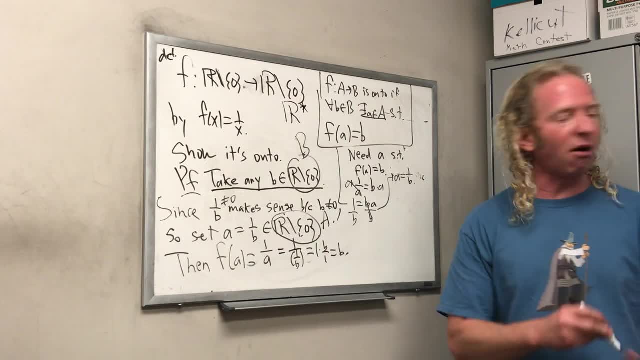 Right, Right. I probably should have said that Right, Like if you were taking a class and someone was grading this, they might look at it and be like, oh, game over, No, They would take points off. So that's what I wanted to talk about today.